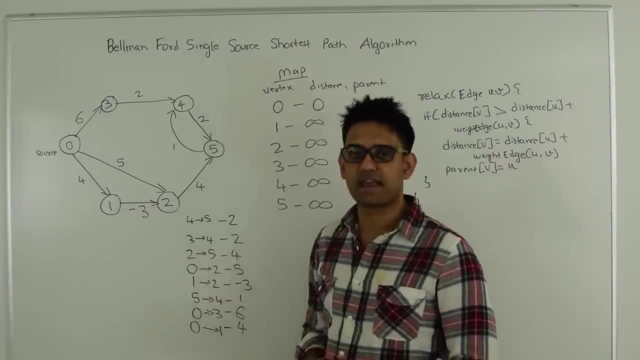 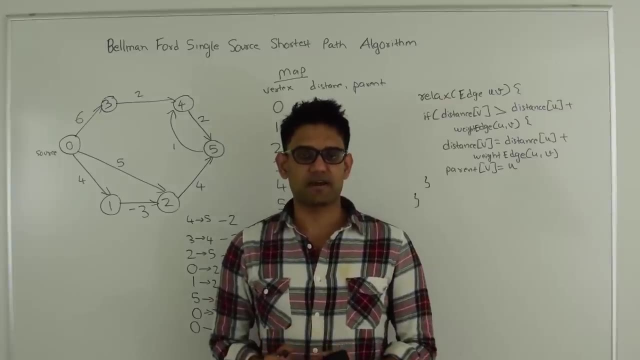 in the cases when the weight of the edge is negative and it also finds negative weight cycles in the graph. So if there is a negative weight cycle in the graph, you cannot find the shortest distance because you can keep going through that cycle again and again and 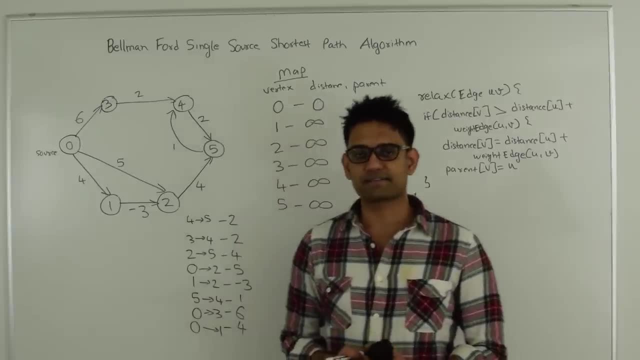 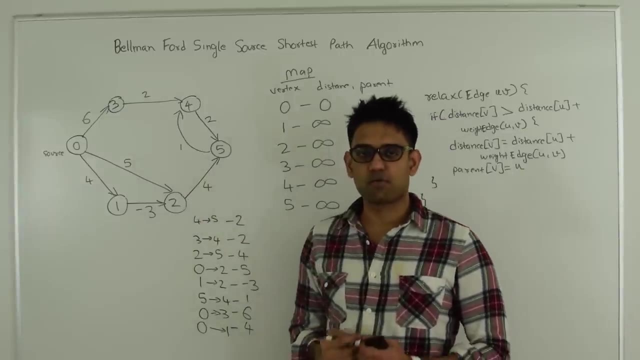 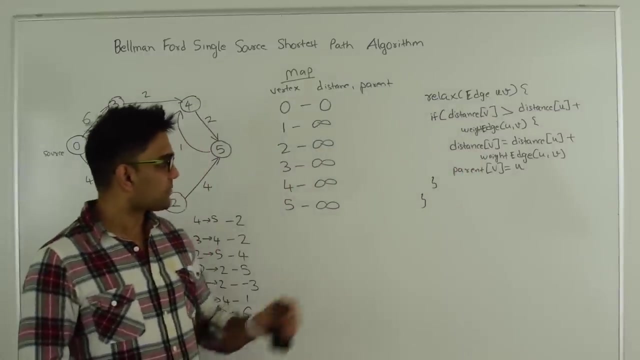 keep reducing the distance between two vertices. So next let's see how Bellman-Ford algorithm works. The idea of this algorithm is to go through all the edges of this graph one by one in some random order. So here I have one random order- it can be any random order- And then apply this relaxation formula on this edge. 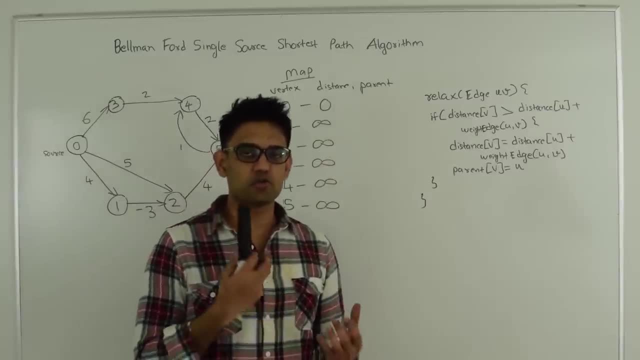 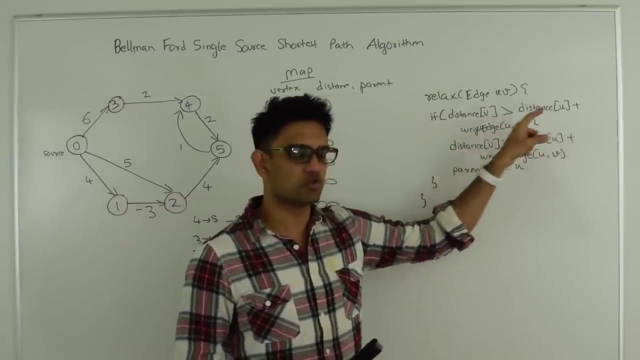 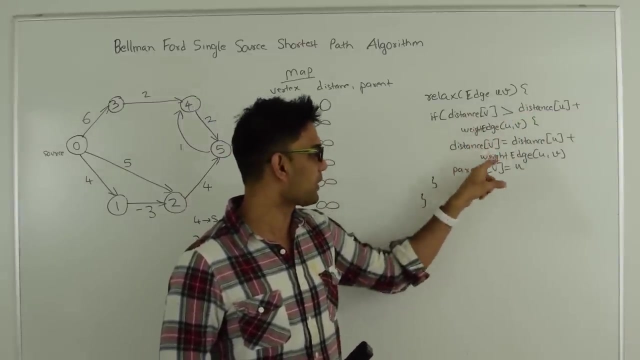 uv. So for given edge uv going from u to v, if the distance to reach v from the source vertex is greater than the distance to reach u plus the weight of edge uv, then you set the distance of v to be distance of u plus weight of uv. 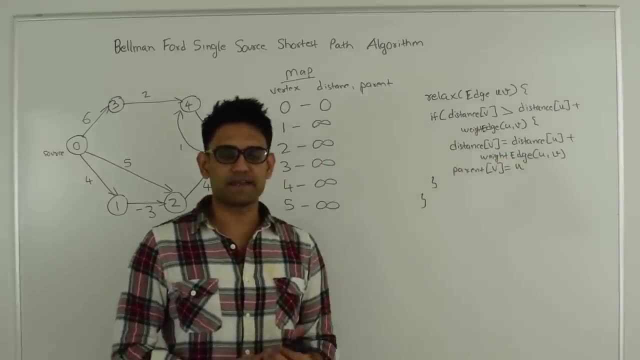 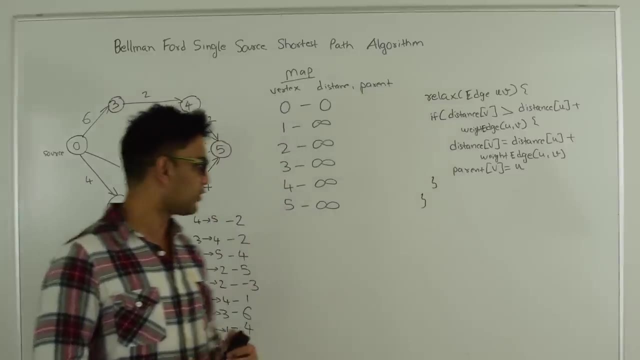 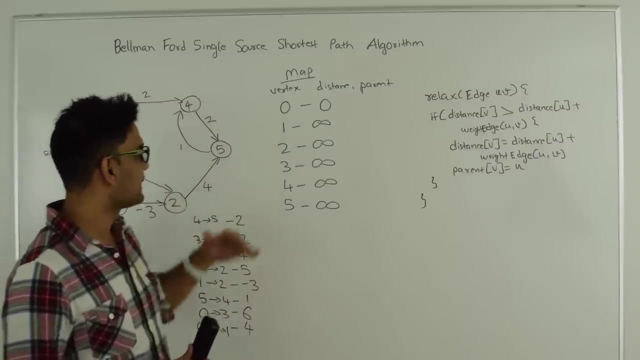 So the distance of edge uv and parent of v to be u And this makes sense. It means that you found another path, another shorter path, to reach v via u, And we are going to store all this information in this map here. So the key in this map are vertex indices and 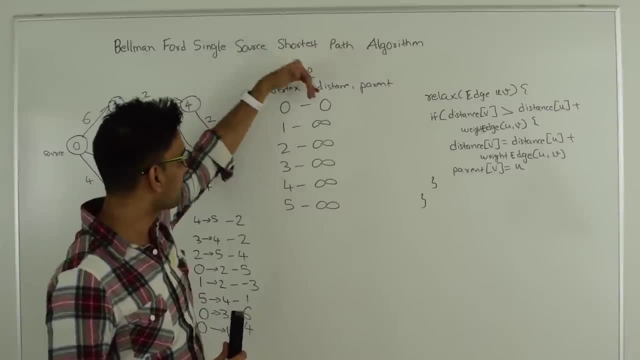 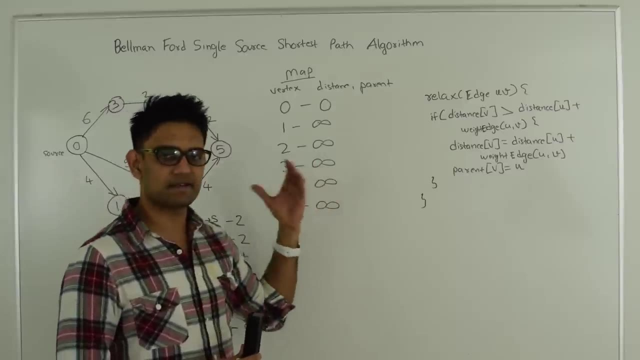 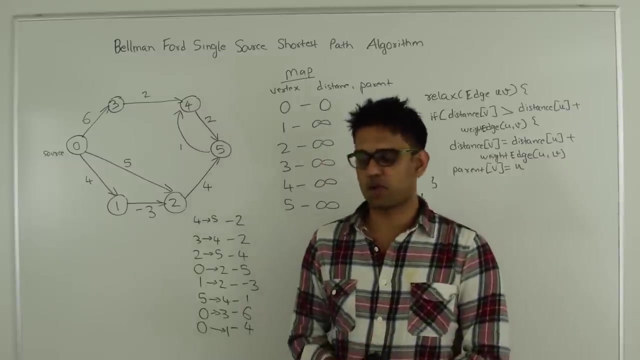 the value in the map is the distance. So the current minimum distance of these vertices from the source vertex and the parent is telling us which vertex it should come through to this minimum distance. So we have to repeat this entire process, v minus 1 times. So we 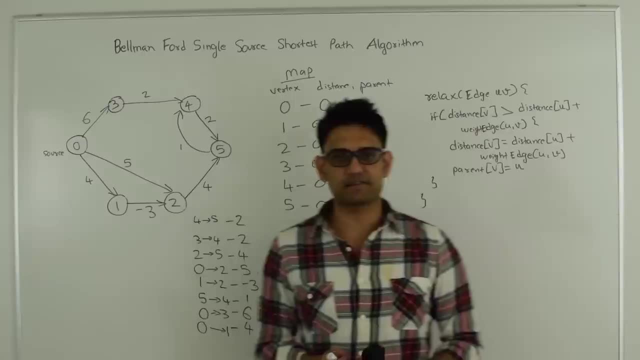 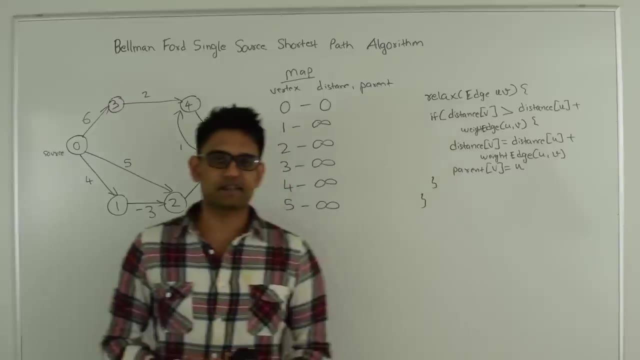 have to go through all the edges and apply this relaxation v minus 1 times. And why v minus 1 times, I am going to tell you at the end of this video. So next let's apply this algorithm step by step on this graph here. 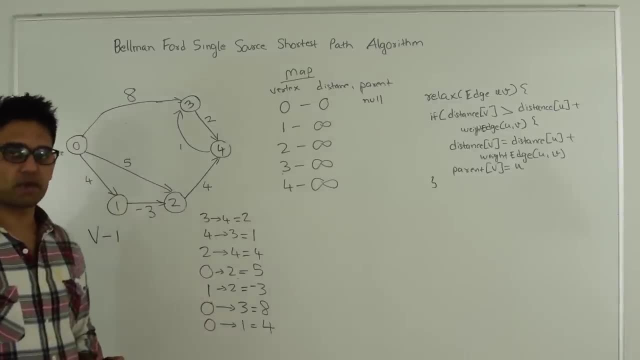 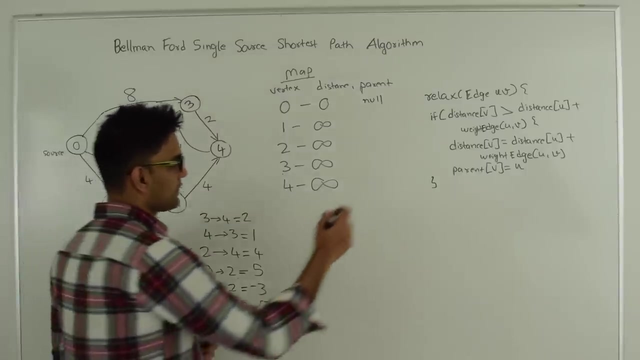 So, as I said before, we go through all the edges one by one, v minus 1 times and apply the relaxation formula. So here we have total 5 vertices. So we are going to repeat this process 4 times. So let's start with edge 3, 4.. So here u is 3 and v is 4.. So the distance of v right now is: 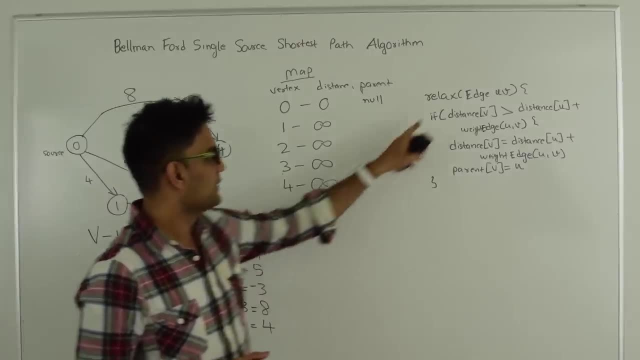 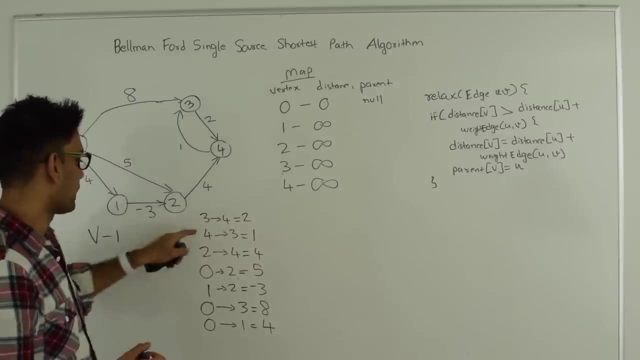 infinity and distance of u right now is infinity. So this if condition will not be true. So this is this edge right now cannot do anything. So let's move on to another edge, 4, 3 which is of, which is of weight 1.. 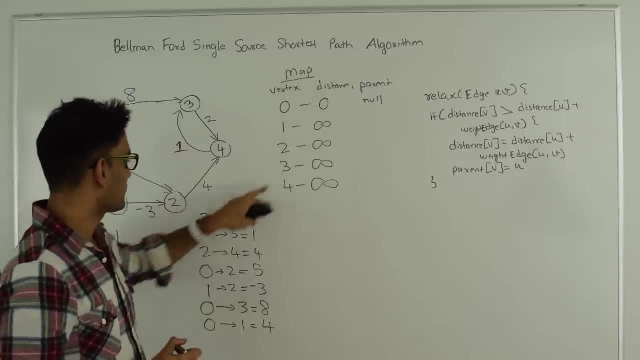 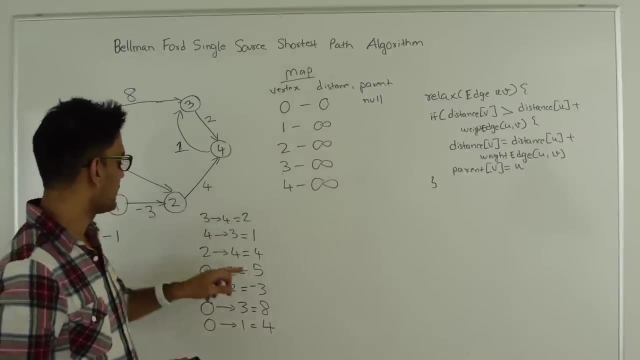 So again, distance of 4 is infinity and distance of 3 is infinity. So this edge cannot do anything. So let's move on to another edge, 2, 4.. Distance of 2 right now is infinity and the distance of 4 right now is infinity. 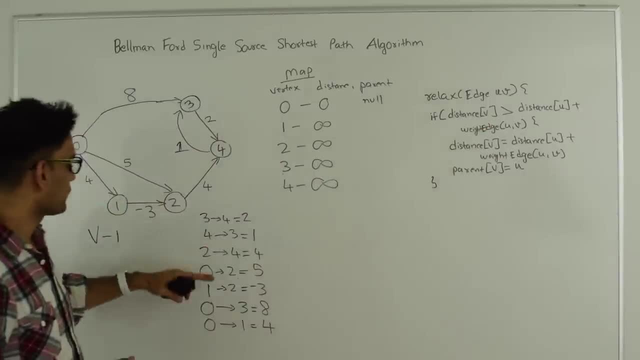 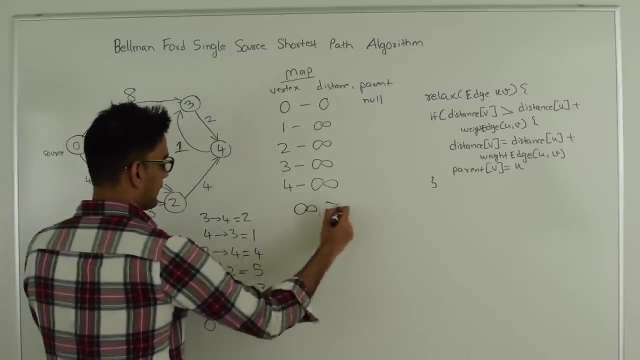 So, again, this edge will not help in this if condition. so move onto the next edge, 0,2.. So right now, distance of 2 is infinity, which is greater than distance of zero, which is zero plus the weight of this edge, which is 4.. 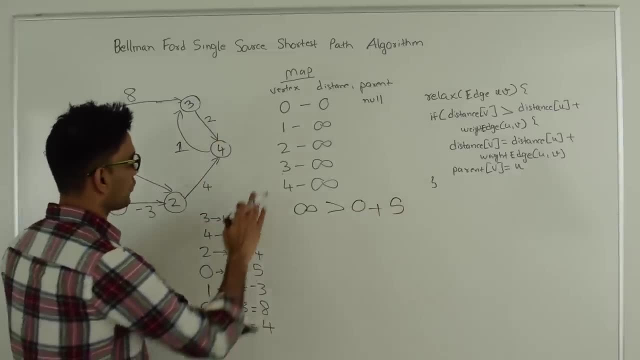 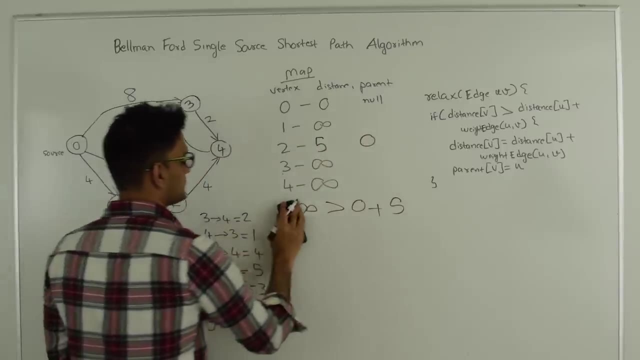 So what we are going to do is we are going to go to 2, update its distance to be 5 and say that it is coming from 0. So, as you can see, as soon as we discovered this edge, we 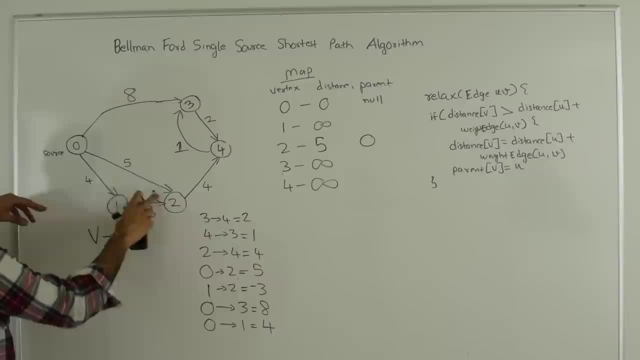 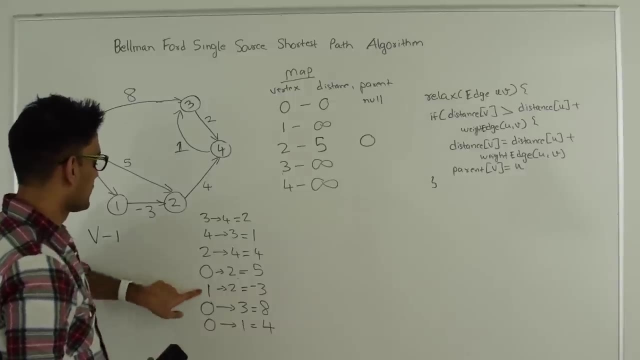 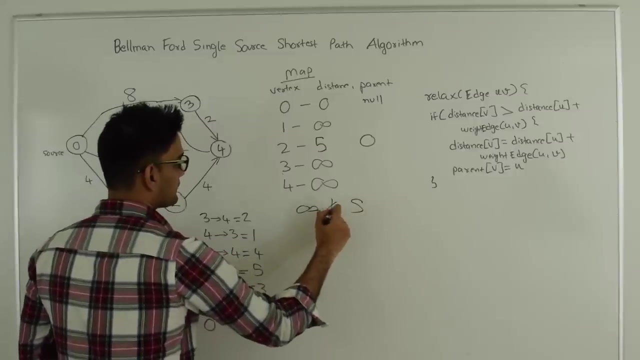 know that 2 is at distance 5 if we traverse via this edge from source vertex 0.. Next we take vertex 1, 2.. So distance of vertex 1 is infinity and distance of vertex 2 is 5.. So this is never going to be the case. So we cannot do anything about this edge. 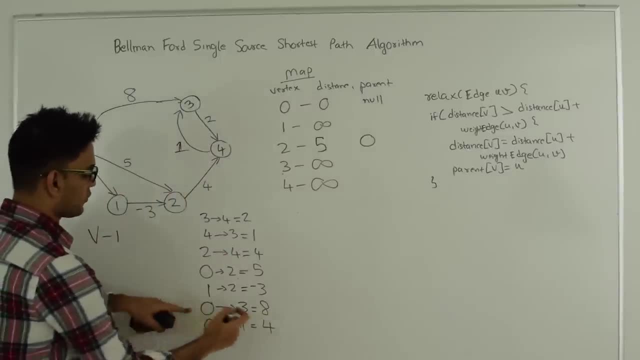 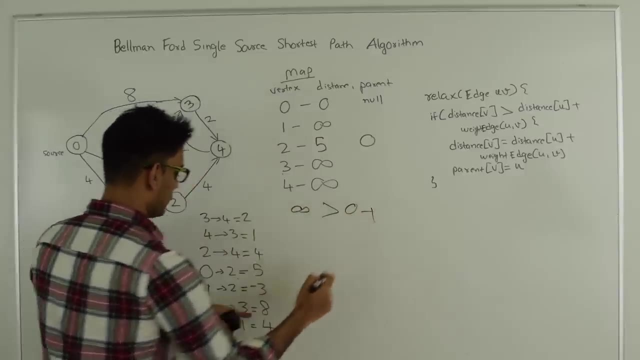 right now. Let's look at edge 0 to 3.. So distance of 3 right now is infinity, which is going to be greater than distance of 0 plus the weight of this edge 8.. So let's update 3.. 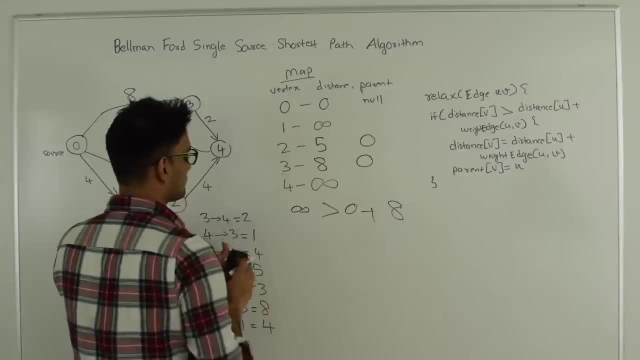 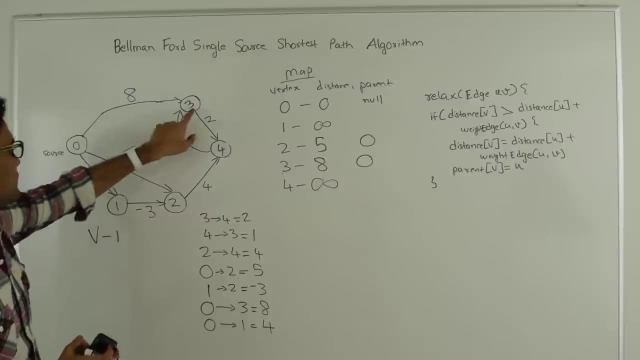 So 8.. And we will say that it is coming from 0.. So again, what happened was we found this edge and we found that 3,, if we take this edge, will be at distance 8 from 0.. And finally, 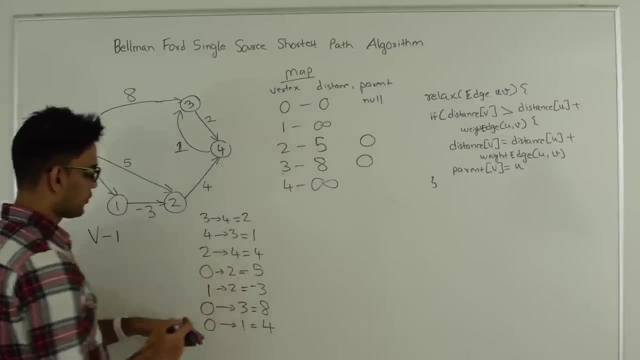 0 to 1.. So, again, distance of 1 is infinity, which is going to be greater than 0 plus the weight of this edge. So this will become 4 and we will say that this is coming from 0. So we found this edge. 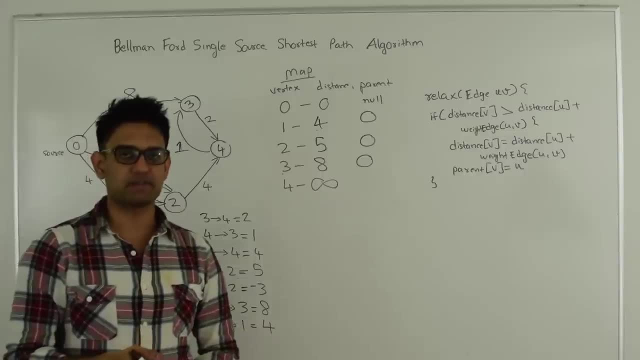 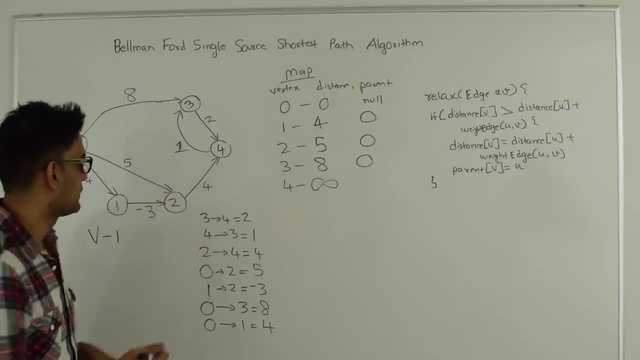 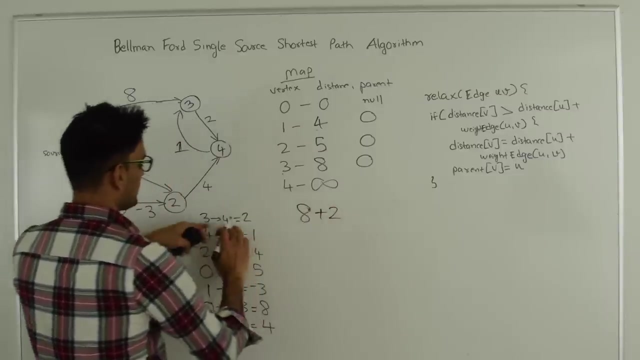 So we repeated this process one time. We have to again, we have to repeat the same process 3 more times. So let's start from here again. So distance of 3 is 8, and distance and plus the weight of this edge is 2.. Weight of this edge is 2 is less than whatever right. 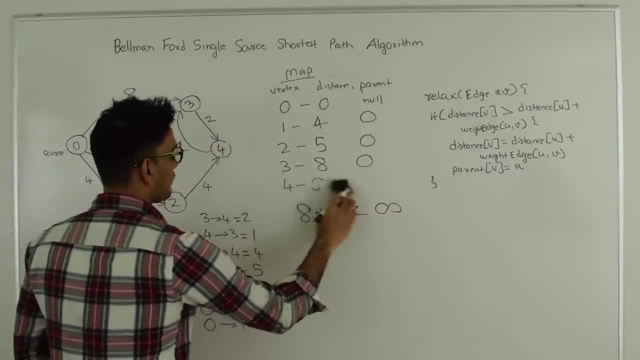 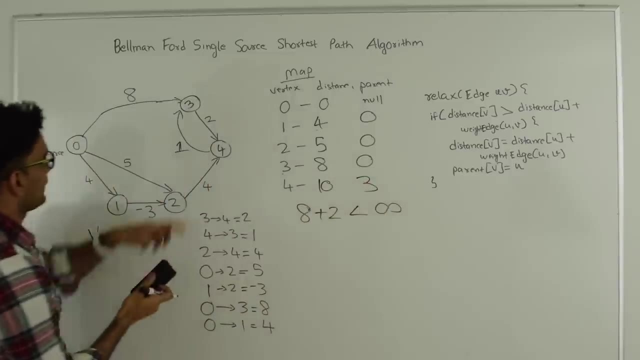 now is with the 4, which is infinity. Yes, So we are going to update this to be this distance 10.. And we will say that 4 is coming from 3.. So, basically, we already found the distance that 3 is at distance 8 and we found this edge. So we know that distance of 4, if we 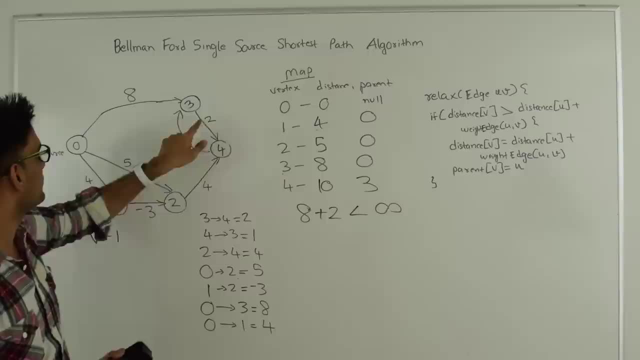 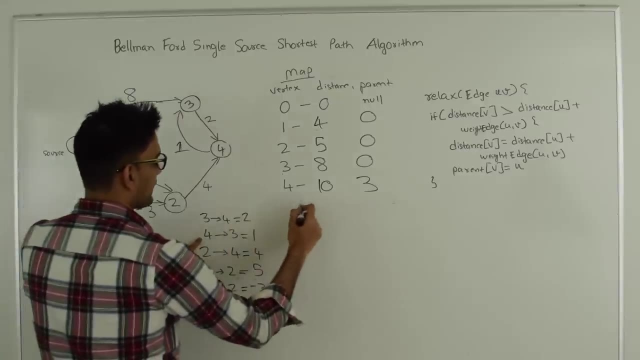 go via this route will be 10, which is this: 10.. 8 plus 2, 10.. So what about 4, 3?? So distance of 4 is 10 and distance of 3 is 8.. So that if condition. 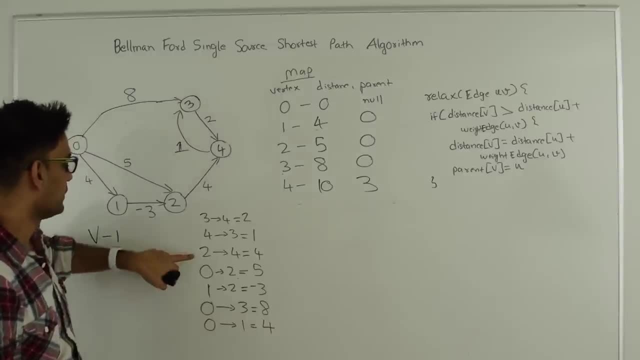 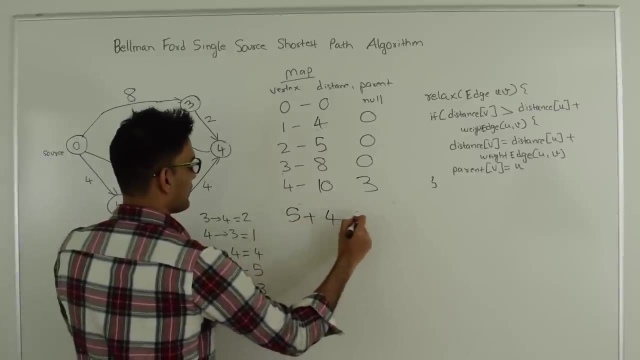 will not be true. So let's pick next edge 2, 4.. So distance of 2 is 5.. So distance of 2 is 5, plus the weight of this edge is 4 is less than the current distance of 4.. So 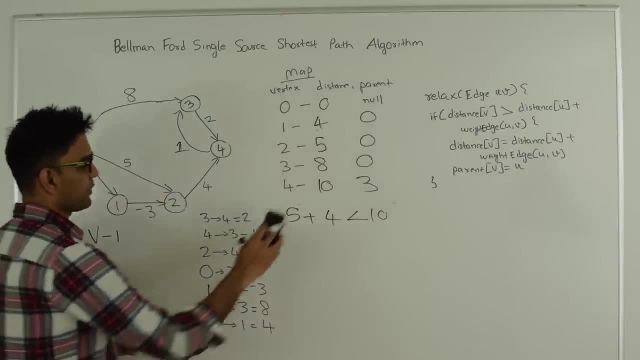 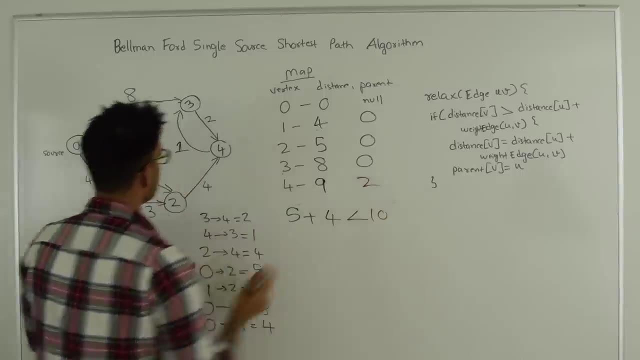 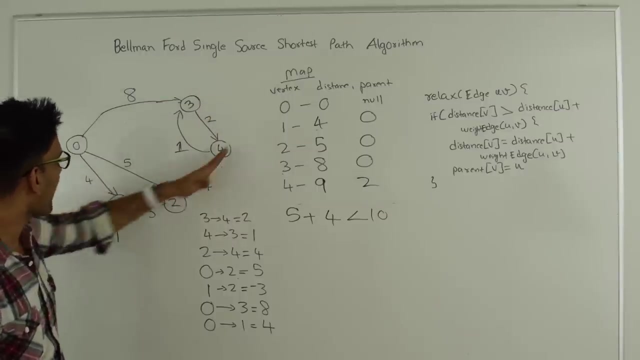 10.. So this is true. So what we are going to do is we are going to update this information to be 9 and we will say that this is coming from 2.. So, basically, what happened was we found one path to reach 4 which was at distance 10, but there is another path to reach 4, which 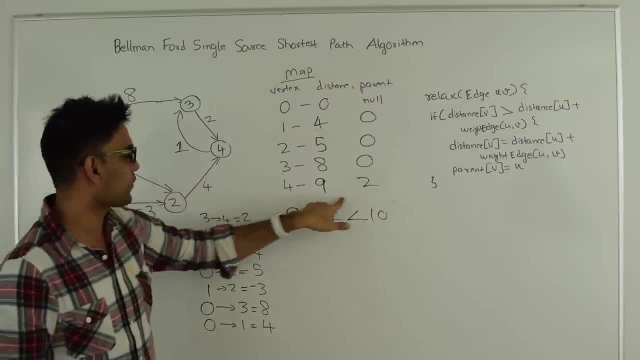 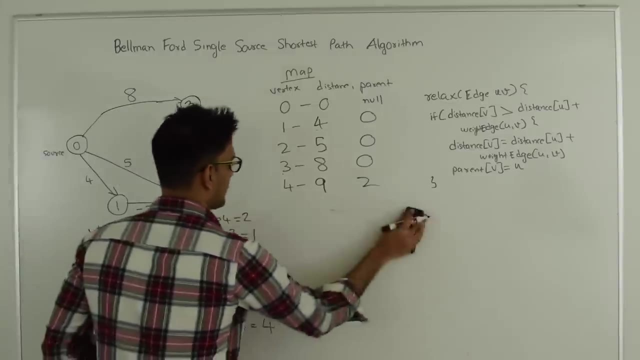 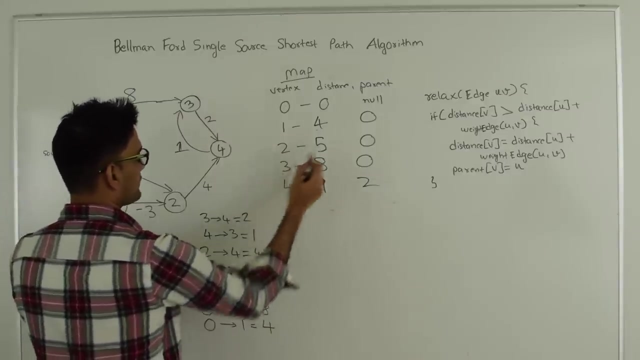 is of distance 5 plus 4, 9.. So that's what we are doing: We are updating this distance and we are saying that now 4 is coming from 2, which is the parent here. Then I am going to pick 0 to 2.. So 0 to 2 is not going to change anything, because 2 is at distance 5.. 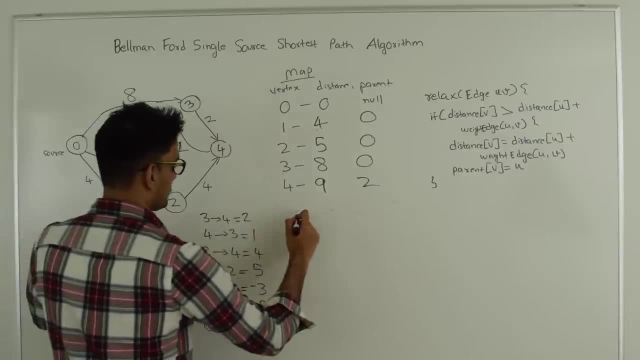 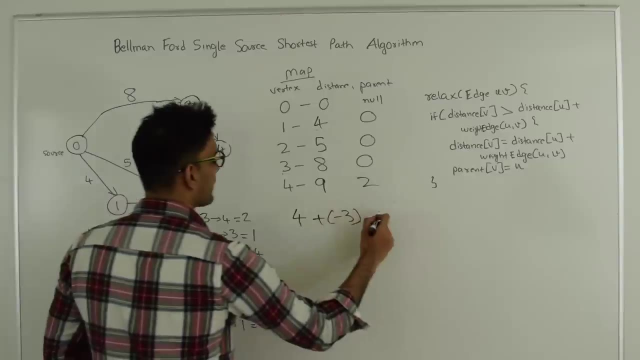 1 to 2.. So the distance to reach 1 is 4 and the weight of this edge is minus 3, and distance to reach 2 is 5.. So this condition is going to be true. So what we are going to do is we are going to. 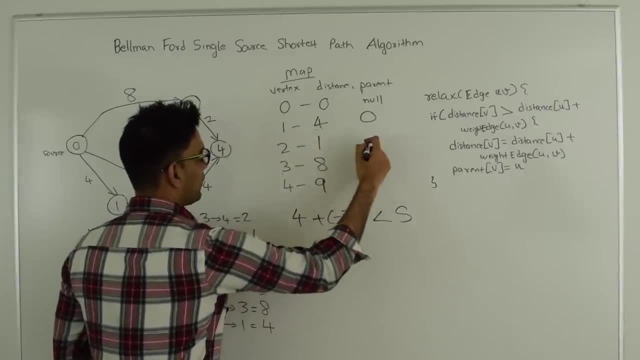 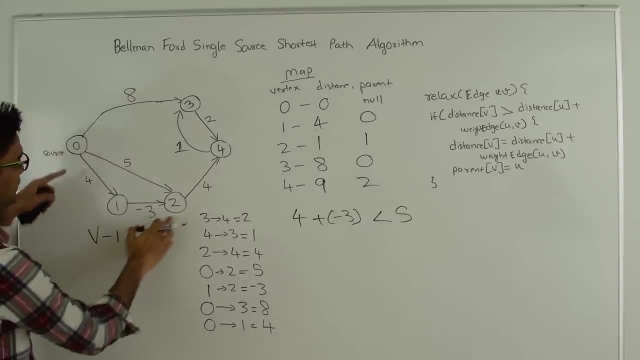 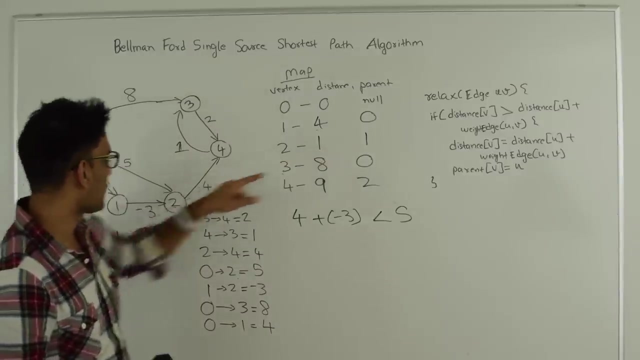 update this distance to be 1 and this also to be 1.. So basically here we found that this edge last time in the last iteration, but we found a shorter path to reach 2, going via 1.. So we update the distance to be 1 through that path and we are also saying that. 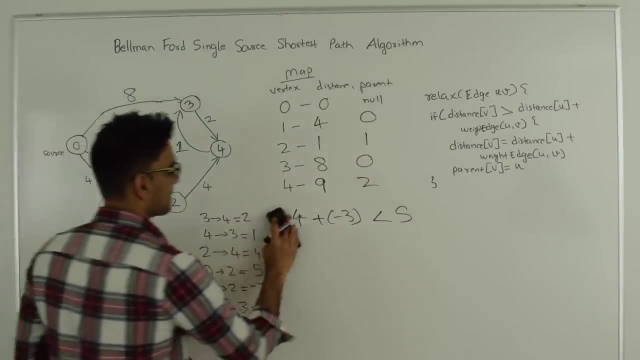 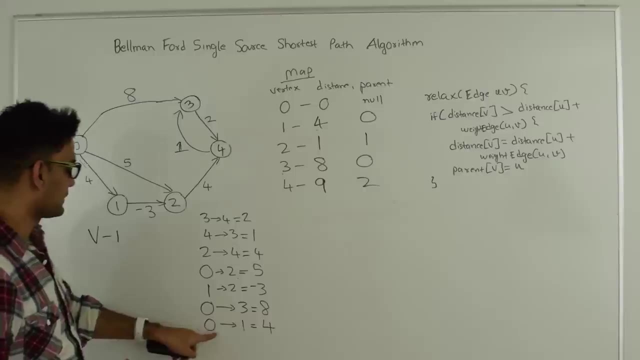 now we are reaching 2 via 1.. And then 0 to 3 is 8, and it's already 8, so it's not going to give us a shorter distance. and 0 to 1 is 4 and it's already 4, so it's not going to give us a shorter distance. 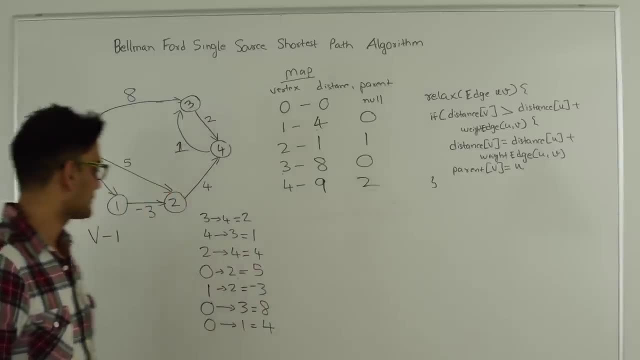 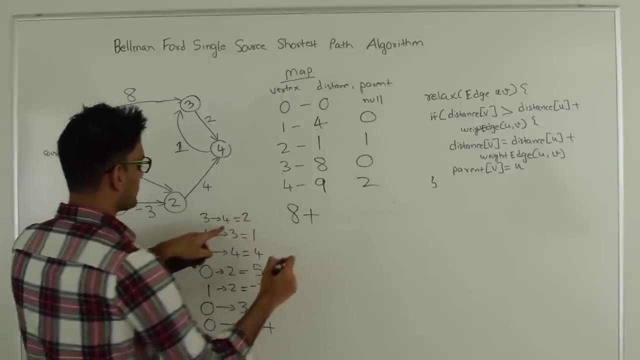 So we did our repetition 2 times. We need to do it 2 more times. So let's pick 3 to 4 again. So distance to reach 3 is 8 plus distance to reach 4 is distance to reach 4, weight of this edge is 2. 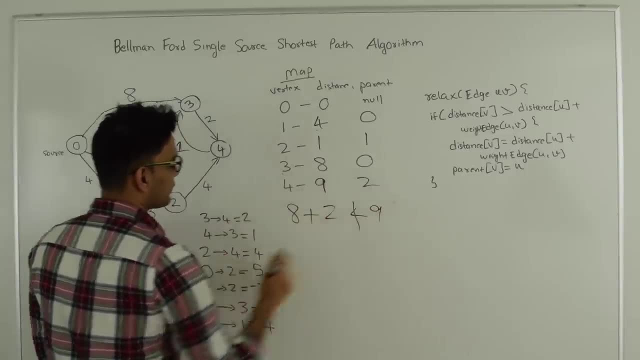 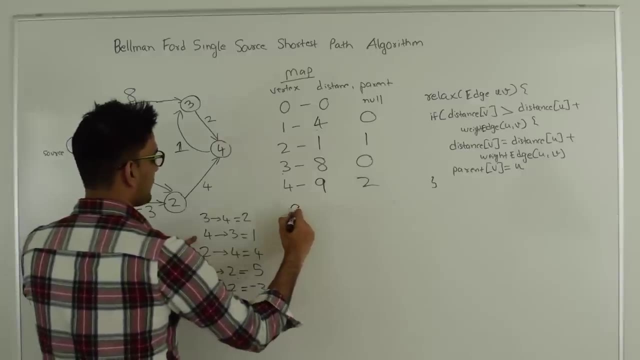 and distance to reach 4 is 9.. So this is not true. So this edge doesn't do anything. yet in this case, What about 4 to 3?? Distance to reach 4 is 9, plus the weight of this edge is 1.. So again, this is not true. 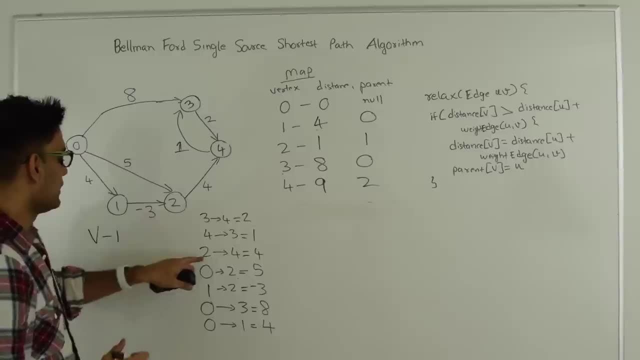 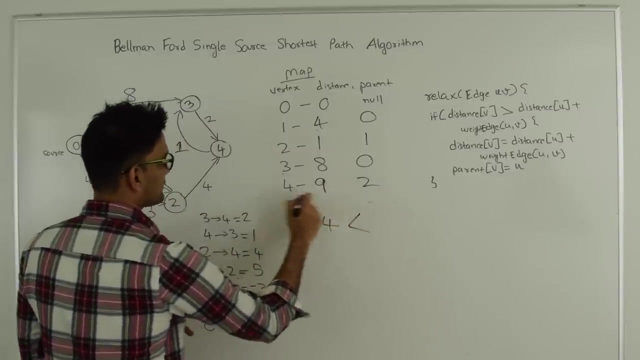 So this edge doesn't help 2 to 4.. So the distance to reach 2 now is 1.. So we can reach 2 in distance 1, plus the weight of this edge is 4. And 4, and the current distance to reach 4 is 9.. So we find a better distance to reach 4.. 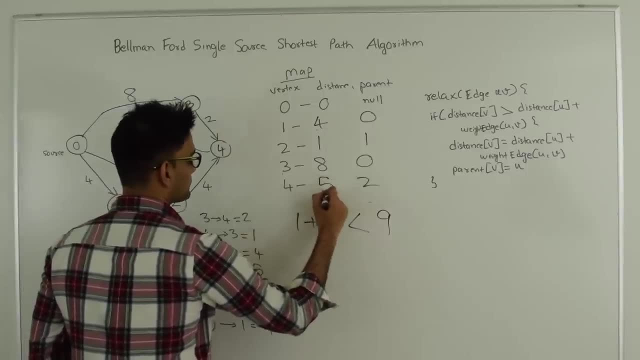 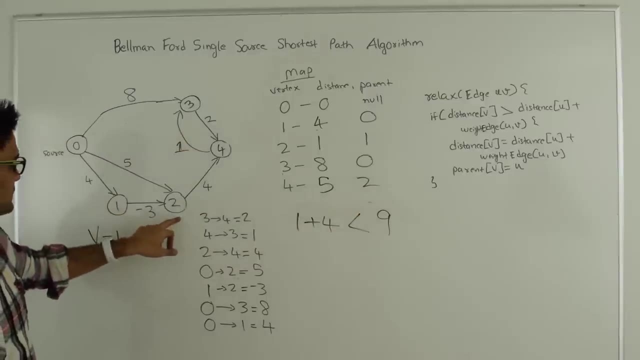 So we are going to update this to be 5.. So last time, when we did a relaxation and then the parent stays, to be 2.. So the last time we did relaxation, the distance to reach 2 was this 5 and with this 4, the value was 9.. 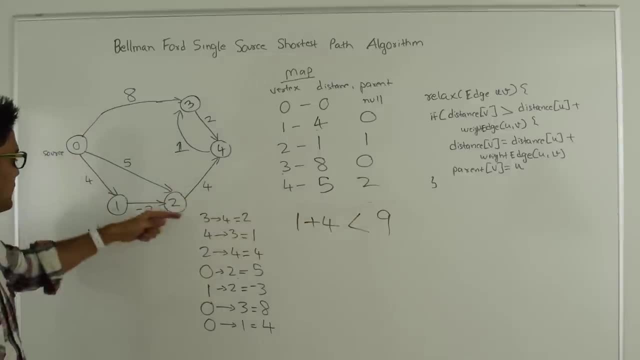 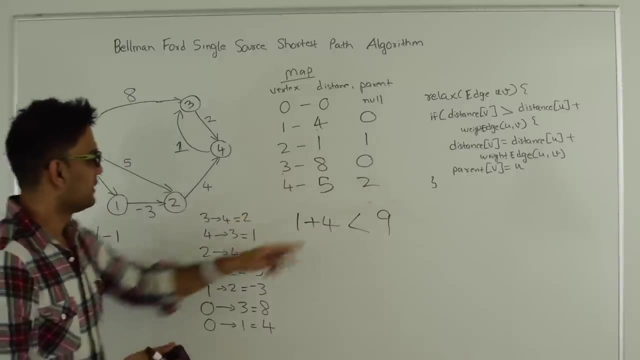 But then we found a shorter distance to reach 2 via 0. And that distance length is 1.. So with that 1 and this 4, now we can reach 4 in total distance 5 going via 2.. 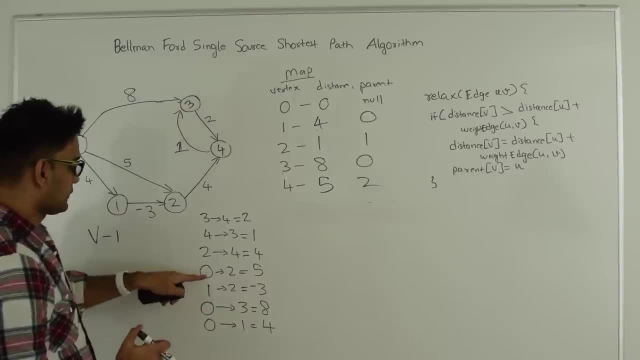 So that was 2 to 4.. Then 0 to 2 is 5 and we already found a very short distance. This is not going to help. 1 to 2 is minus 3 and we are already at the shortest distance with 2.. 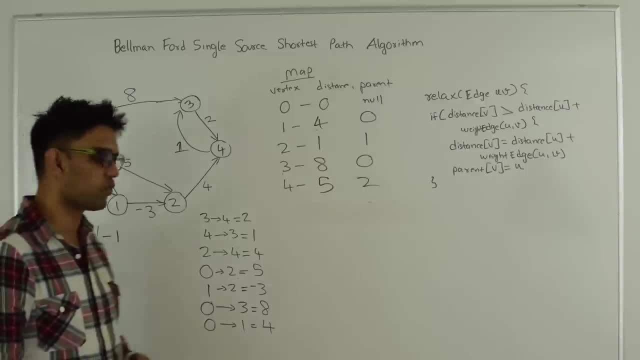 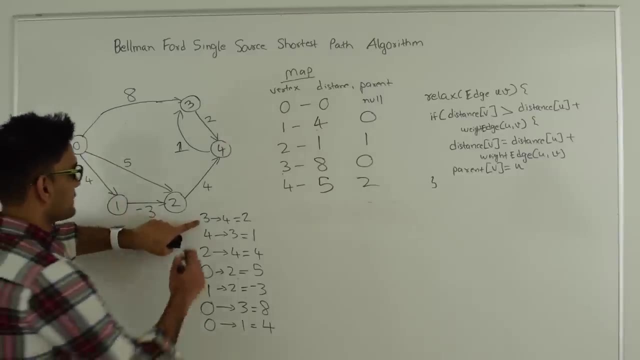 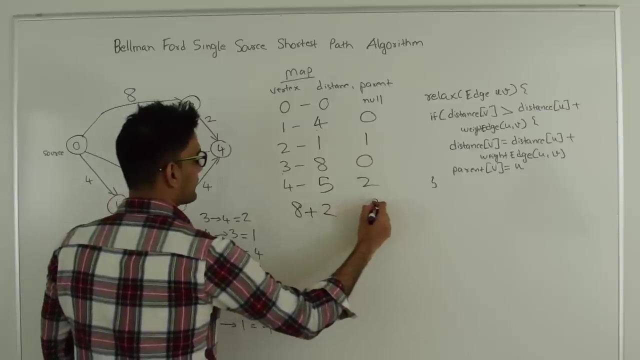 This is not going to change anything. 0 to 3 is not going to change anything and 0 to 1 is not going to change anything. So we are done with 3 repetitions and we have to do one more repetition. So, again starting, the distance to reach 3 is 8 and plus the weight of this edge and distance to reach 4 is 5.. 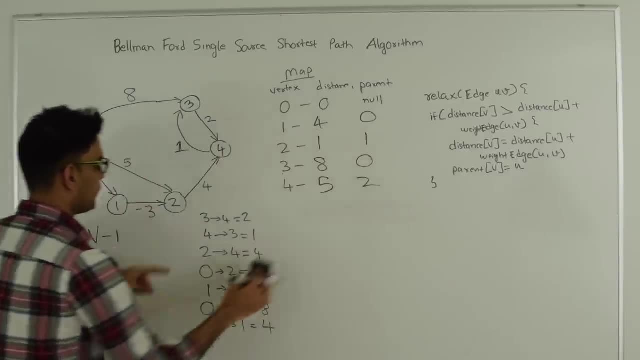 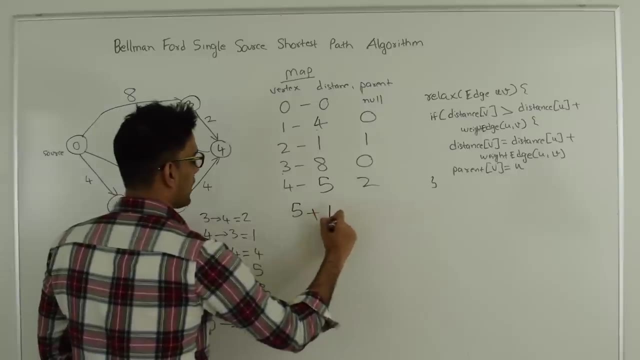 So this is not true. So this edge cannot help. Moving on to the next edge, distance to reach 4 is 5 plus the weight of this edge is 1.. And this is less than the current distance to reach 3, which is 8.. 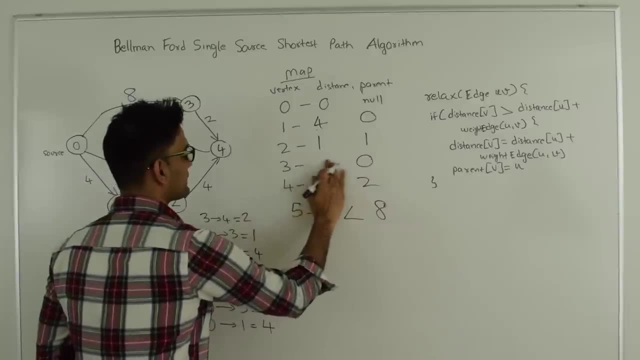 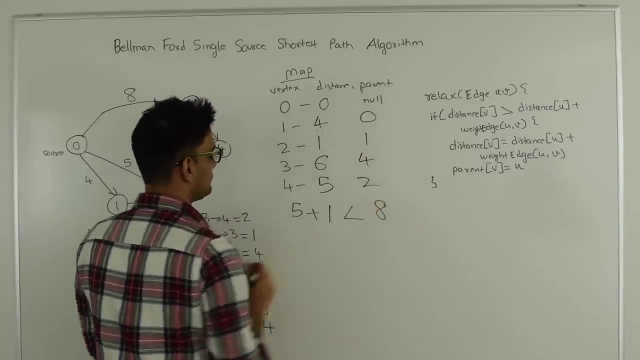 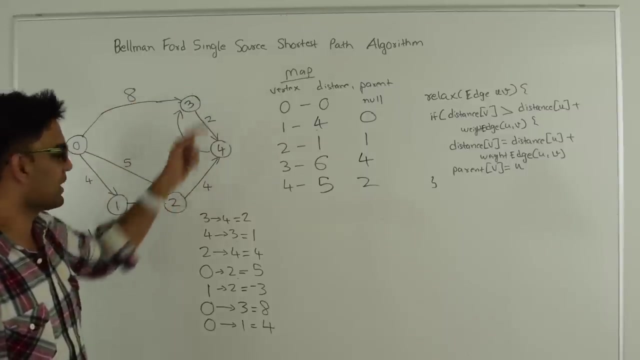 So we found a shorter distance to reach 3, and that distance is 6.. And now we are coming from this vertex 4.. So now we found a shorter distance to reach 3, which, instead of going from 0 to 3, we can come via this route here. 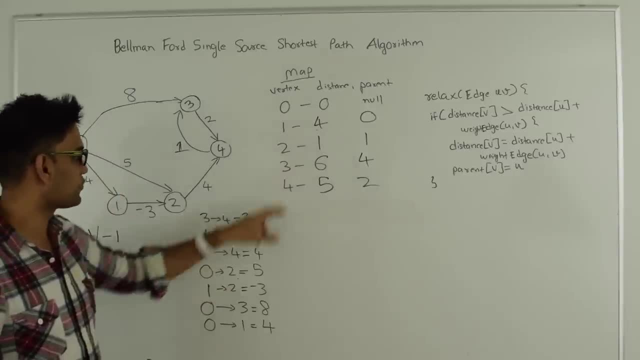 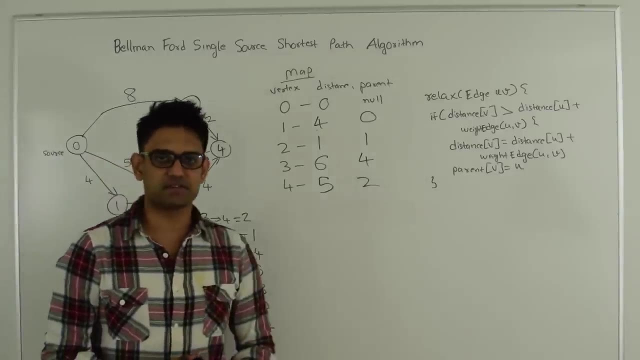 And then 2 to 4 is not going to change anything, 0 to 2 is not going to change anything And rest of the other edges are also not going to change anything. So we have done 4 repetitions of this graph here and we found the shortest distance. 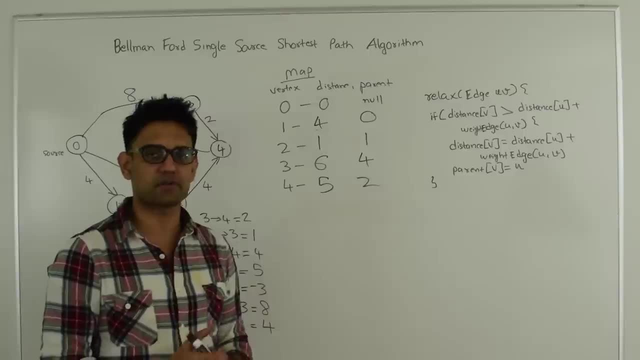 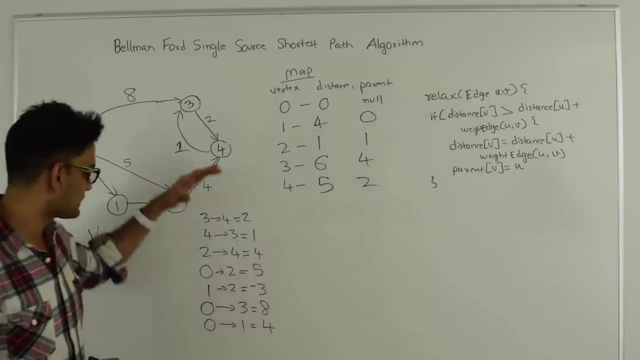 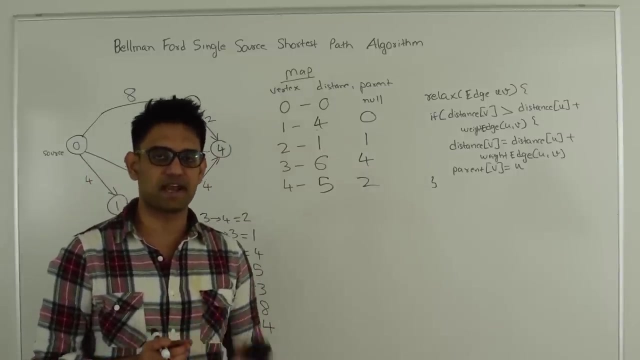 And we also found the how to reach the. what is the path for the shortest distance. So after we are done doing V minus 1 repetitions, we do one more repetition with the same edges, And if it reduces the distance even more, it means that there is a negative weight cycle in the graph. 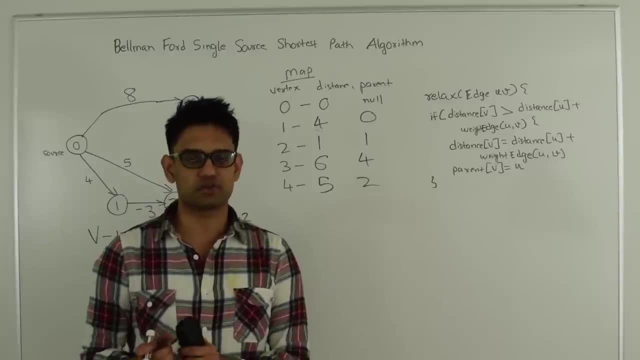 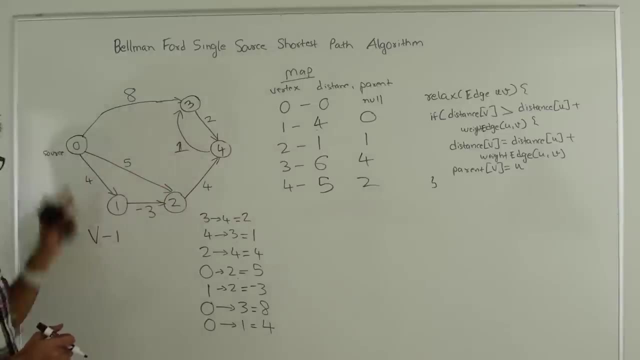 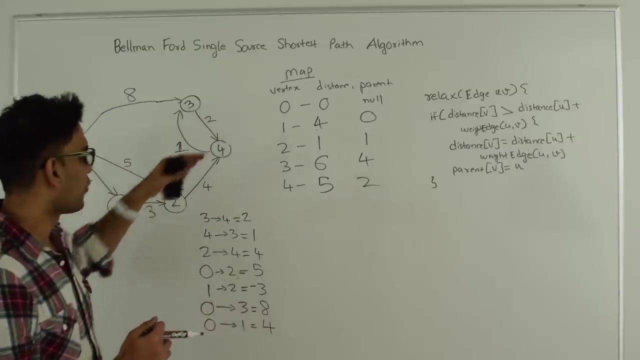 And I am going to show another example to show that, show how that works. But in this case, going through this again is not going to change anything because there is no negative weight cycle in this graph. So finally, let's see: how do we find what is the path to reach a vertex from the source vertex. 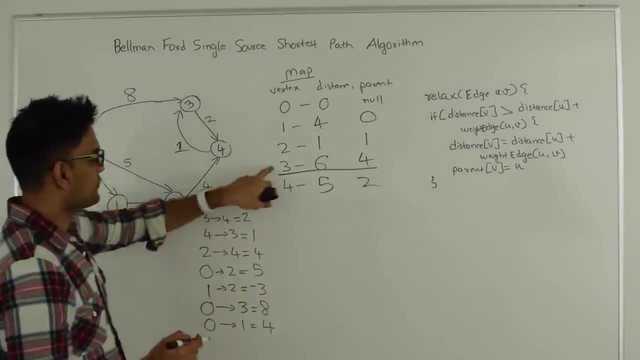 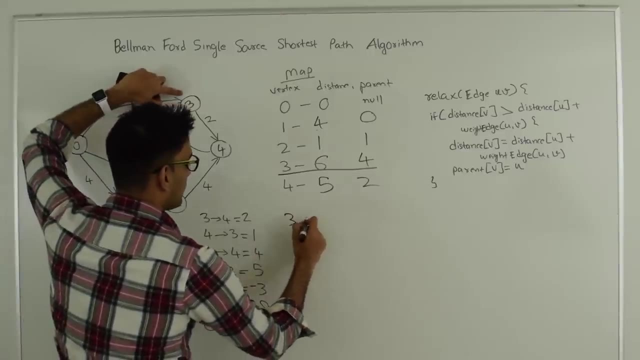 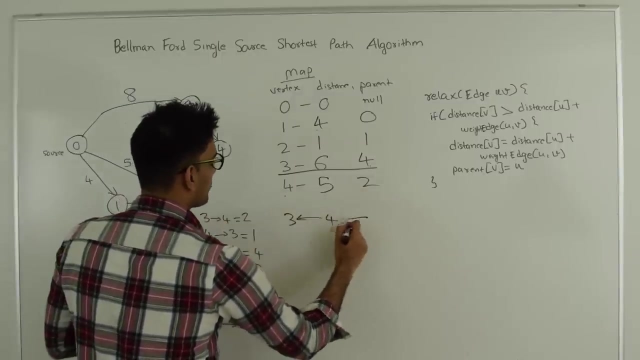 So let's look at this example here. So to reach 3, we know that it is coming from 4.. So we know that 3 is coming from 4.. Okay, So then we go to 4 and jump here, and we know that 4 is coming from 2.. 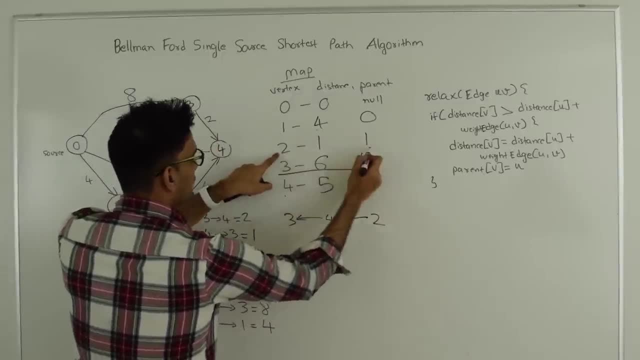 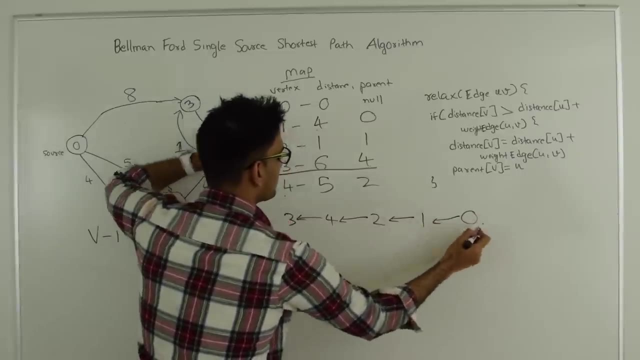 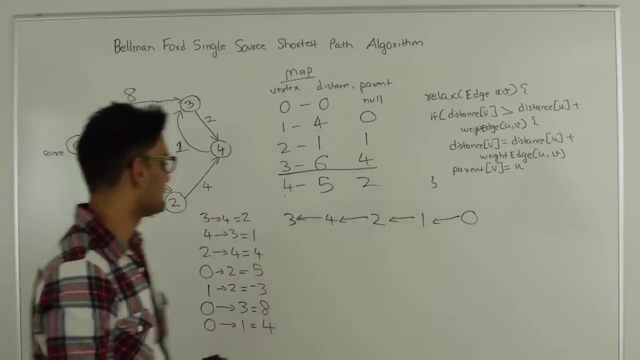 Then we go to 2 and we know that 2 is coming from 1.. And then we go to 1 and we know that 1 is coming from 0 and 0 is our source vertex. So this is the path to reach. this is the shortest path to reach 3 via 0.. 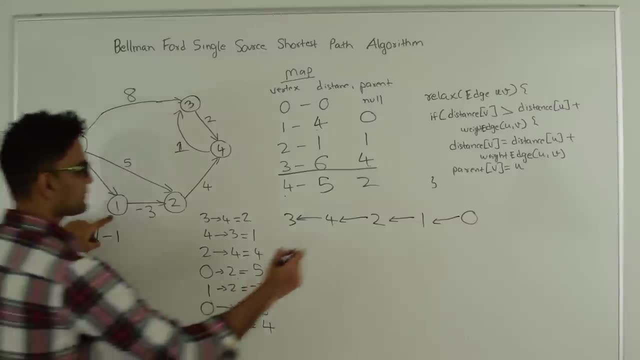 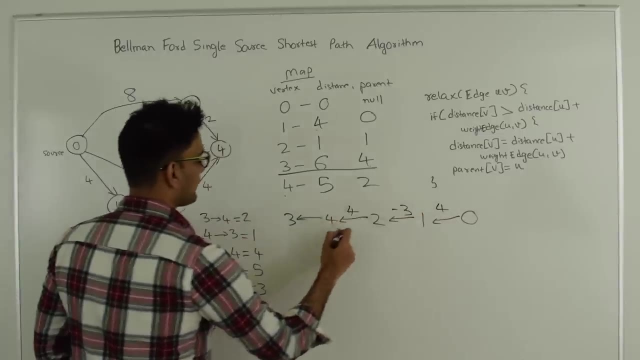 And let's see that. So 0 to 1 is 4.. 1 to 2 is minus 3.. 2 to 4 is 4. And 3 to 4 is 1. So the total distance here is 5 minus 3.. 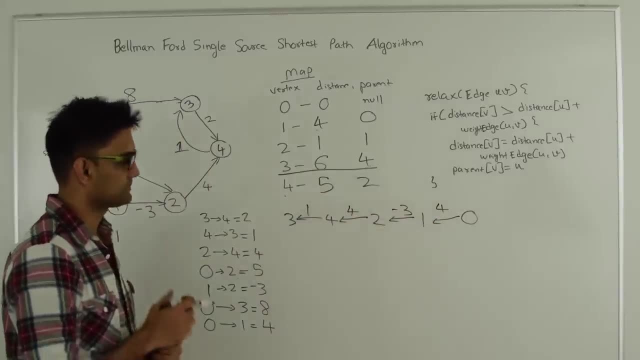 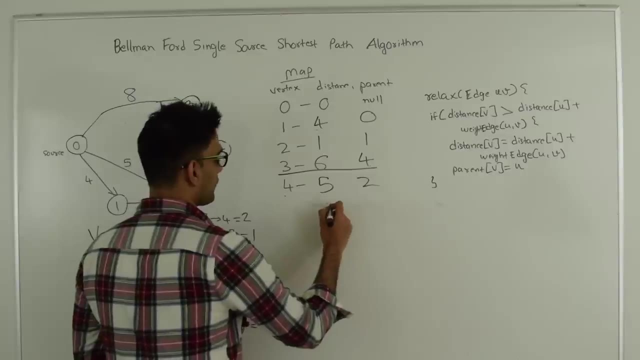 2 plus 4 is 6. which is this distance here? Let's quickly analyze the time complexity. So the time complexity of this algorithm will be O of V into E. So it's pretty clear. We are going through all the edges. 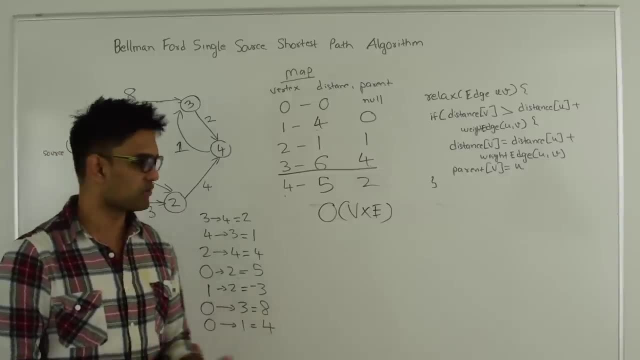 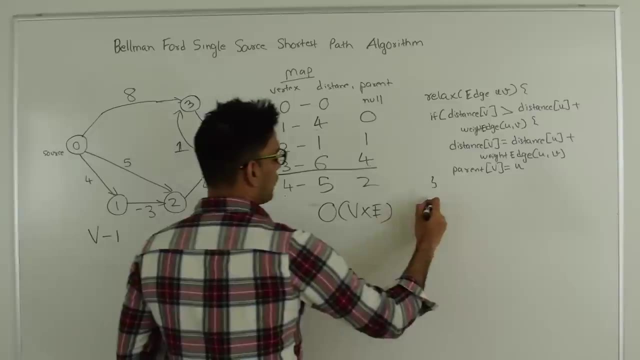 V minus 1 time and at the end we go one more time to see if there is negative weight cycle. So the time complexity is O of V into E, The space complexity is O of V. We can also use this algorithm to find all pair shortest paths. 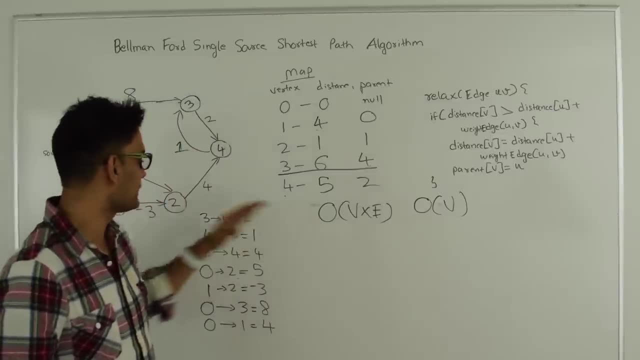 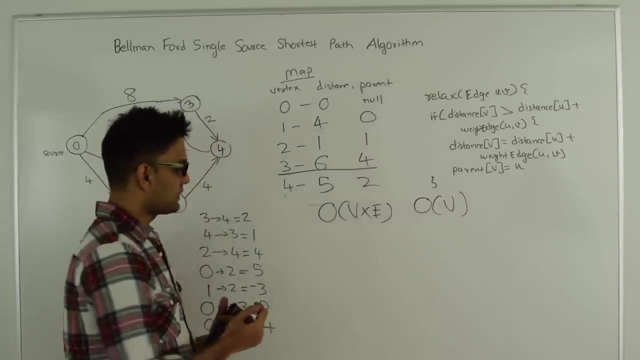 So basically the shortest path between all the pairs. All you have to do is repeat this process for considering all the other vertices as a source vertex. In that case, for all pair shortest paths, the time complexity will be O of V square into E. 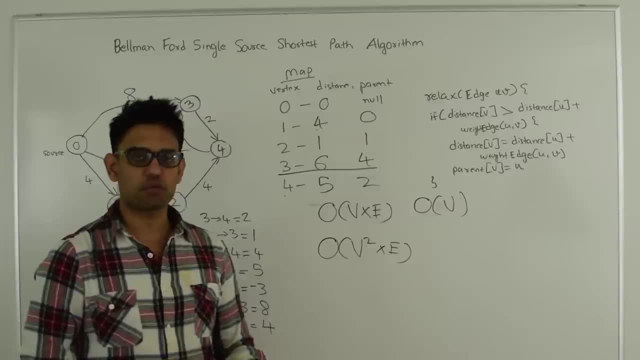 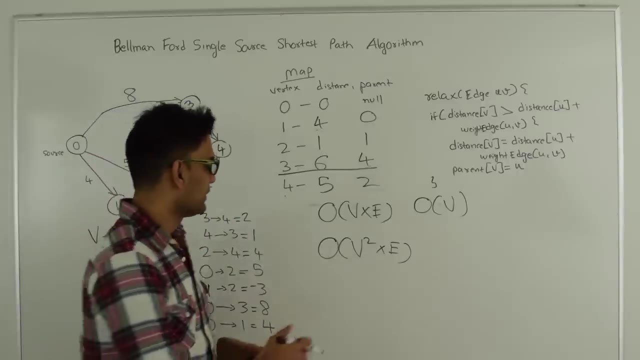 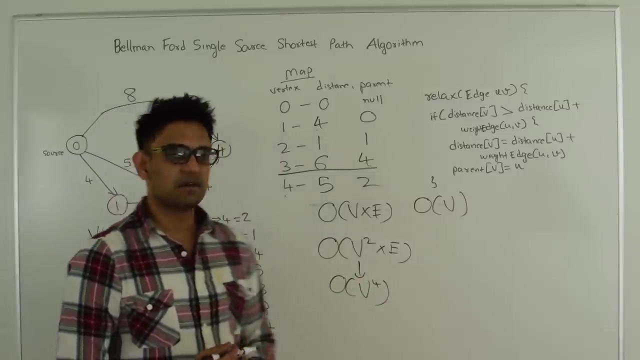 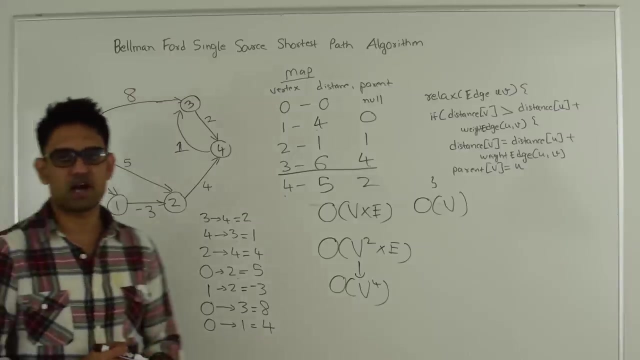 But there are faster algorithm than this, like Floyd-Warshall algorithm, which does it in O of V, cube time, And here, in the worst case, E could be V square, So this could really be O of V raise to 4 time. So next let's try to understand why we are repeating this process: V minus 1 time. 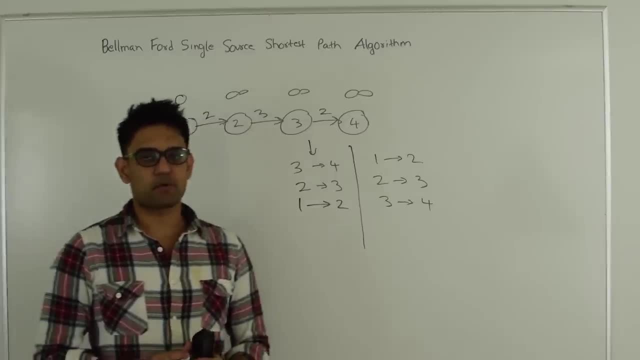 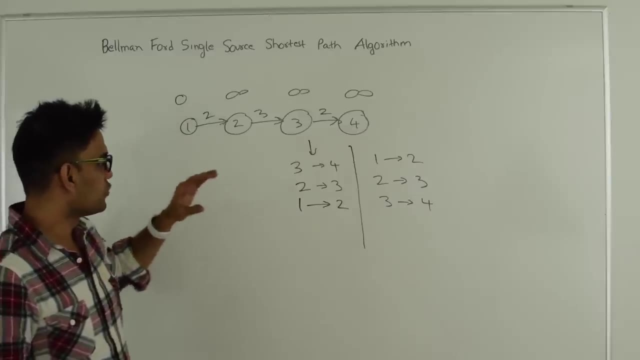 Let's try to understand why we need to repeat the process V minus 1 times. So if you look at this graph here, if the source vertex is 1, to reach 4, in the worst case it will take V minus 1 edges. 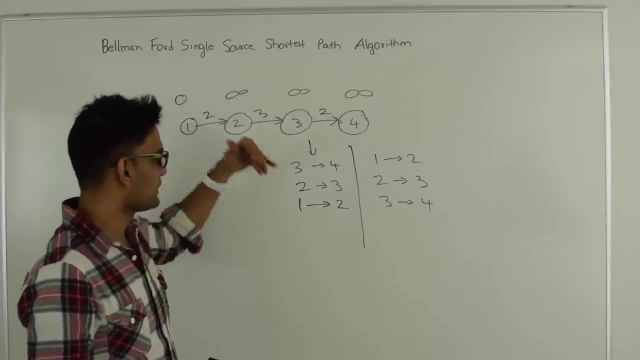 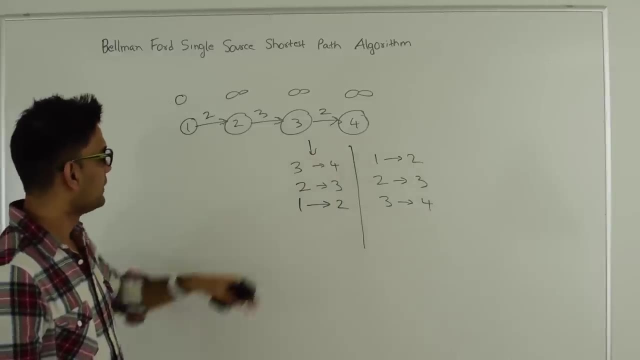 So now, depending on the order in which the edges are discovered, it might takes V minus 1 times to discover 4.. So let's look at this simple example. So if we try to relax 3,, 4,, it's not going to change anything because 3 has not been discovered. 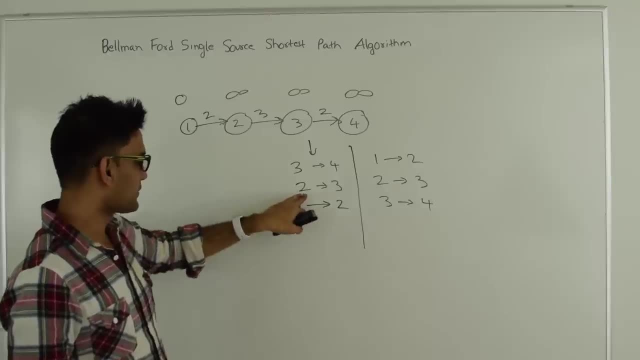 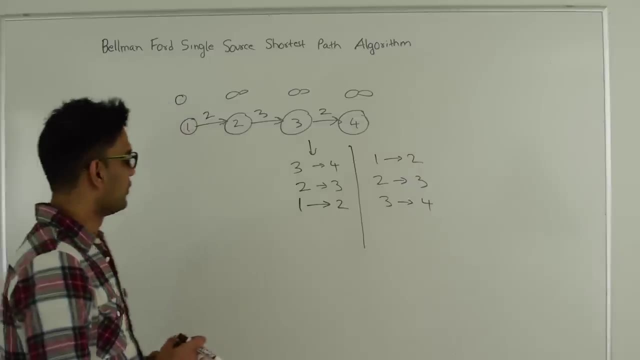 and the distance of 3 is infinity. Then we try to pick edge 2, 3, and it's also not going to change anything because 2 right now is also infinity. Then we go to 1, 2, and 1 is a distance 0 with itself. 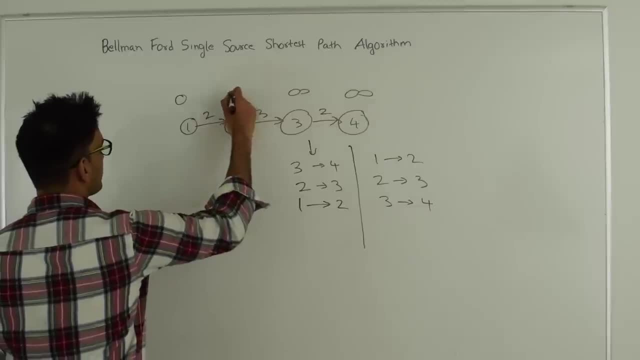 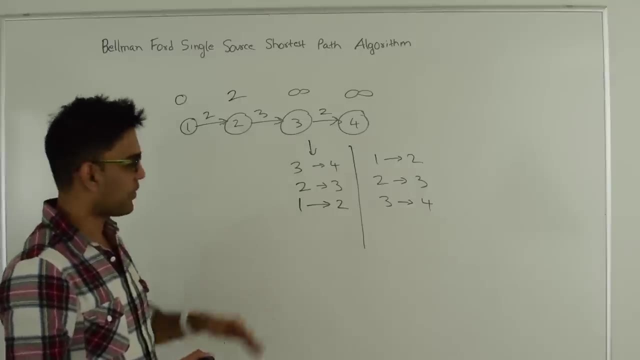 So we discover 2 now, So this distance becomes 2.. So we discover 2 after first iteration, how far it is from 1. Then we go back and repeat the same process, So 3 is still not discovered. 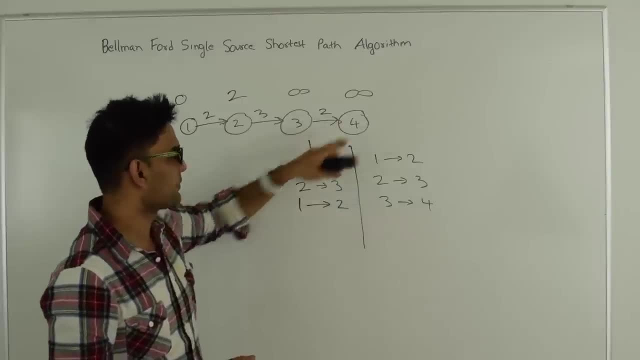 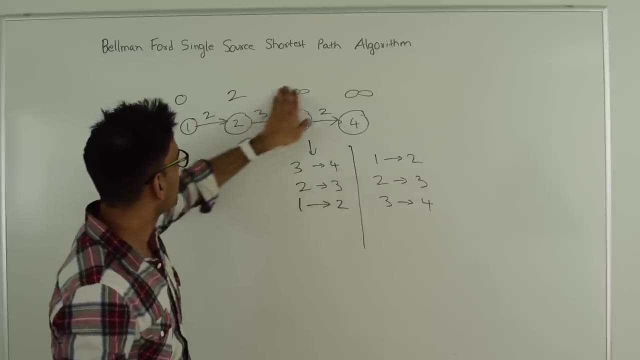 So we don't know what is the minimum distance to reach 4.. And now we go to the second edge: 2, 3.. Now that 2 has been discovered, we know that 3 is a distance whatever is at 2 plus 3, so 5.. 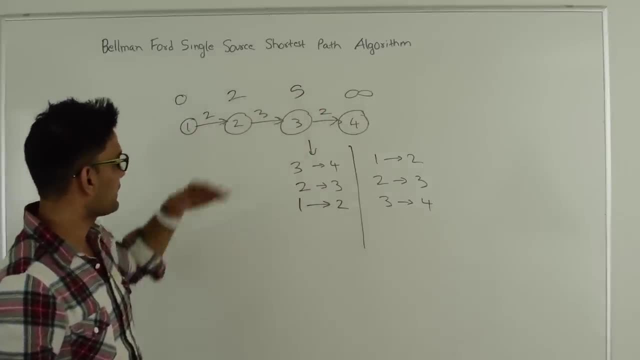 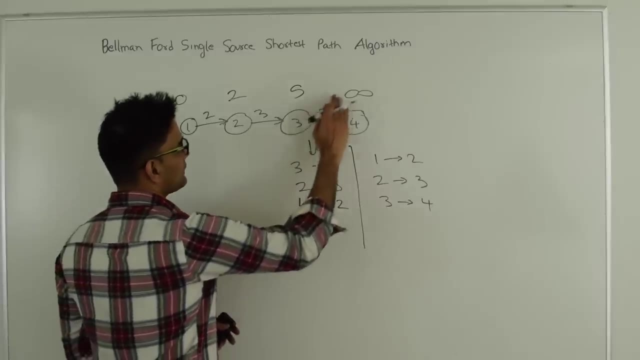 And then 2 is already discovered. And then we go back to the top again, and this time now we know that how far 3 is from 1, source vertex. So we know that 4 will be that distance plus 2, so that is 7.. 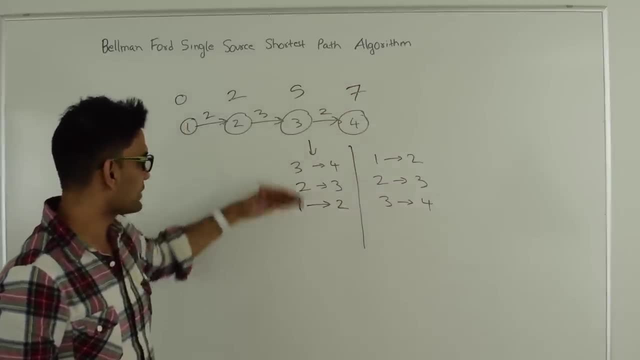 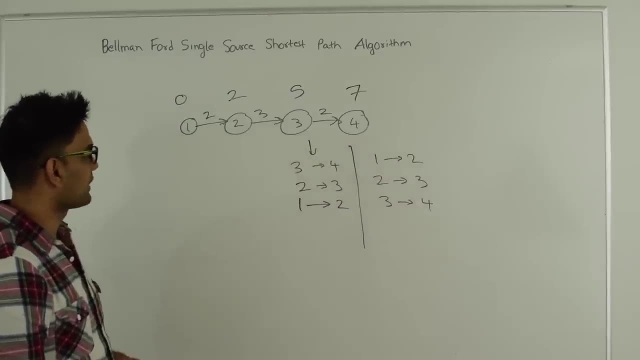 So, as you can see, it took me 3 iterations of going through these edges again and again to find out how far 4 is from the source, vertex 1.. And the worst case here would be that, since there are 3 different, 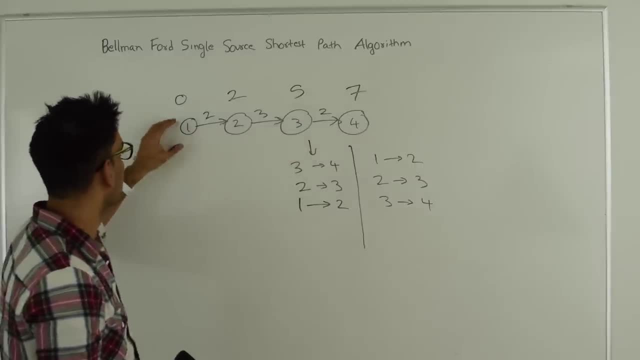 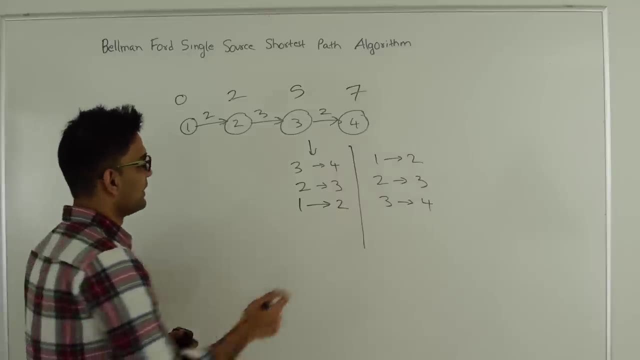 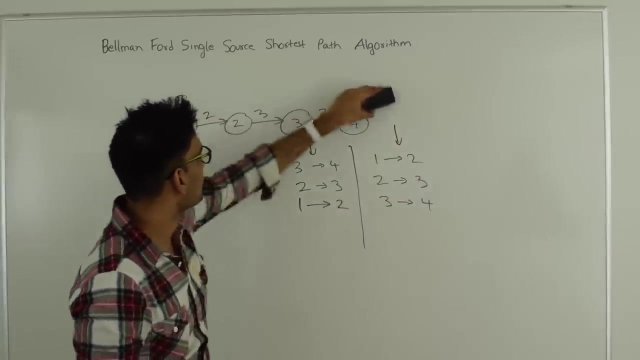 since there are v-1 edges from source vertex to the last vertex, we have to repeat this process v-1 times. If we had, if we had picked edges in this way, in that case we would have found the result in one iteration. 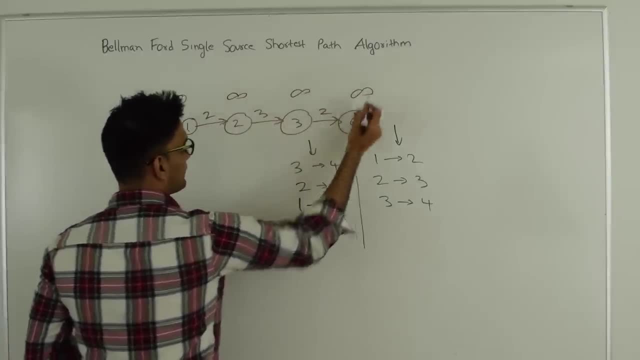 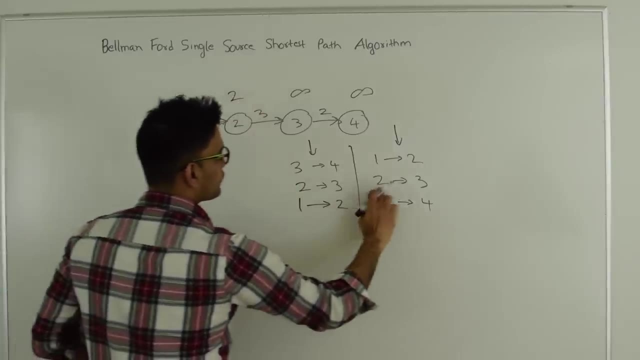 So if this is infinity, this is infinity, this is infinity. So 1 to 2, so we find how far 2 is from 1, which is 2.. Then we go to 2 to 3.. So this helps me relax. 3. 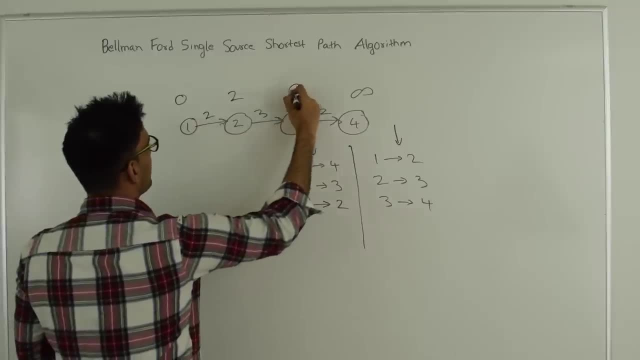 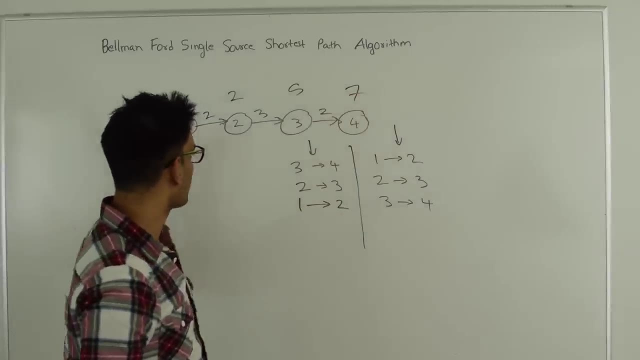 because we already know, distance of 2 is 2 plus 3, 5, which is less than infinity, And then 3 to 4, this will become 7.. So if we had picked edges in this way, we could have found. 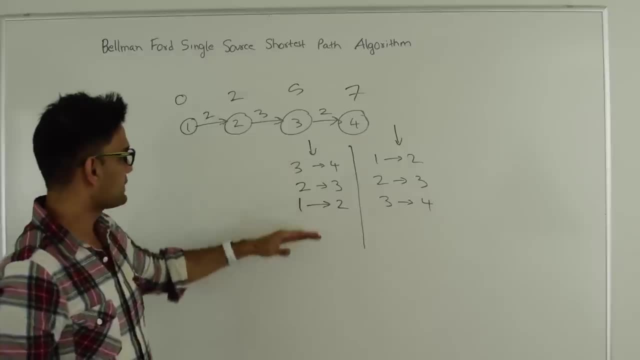 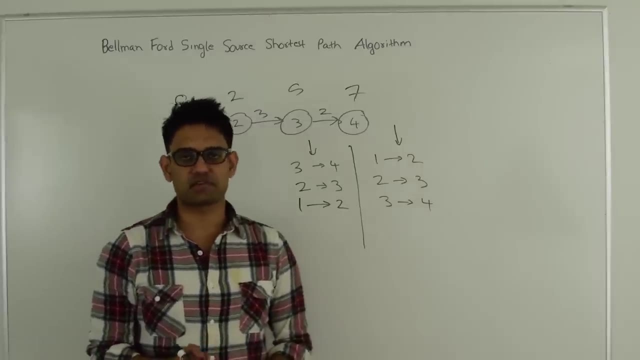 we could have solved it in one iteration, But in the worst case it will take 3 iterations, which is v-1, and which is why we are repeating this process v-1 times. Next, let's look at an example of how. 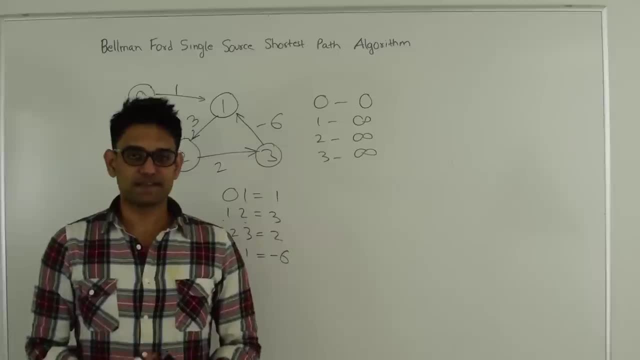 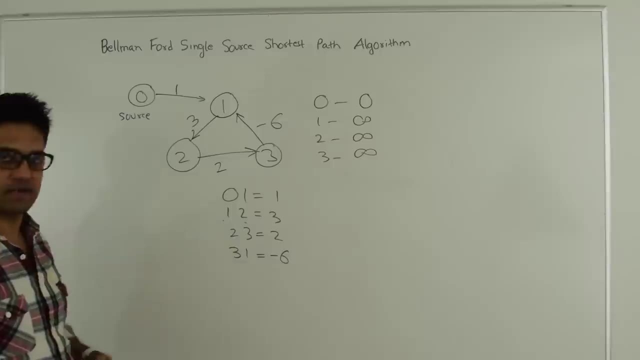 what happens if there is a negative weight cycle in this graph. So let's see how Bellman-Ford deals with negative weight cycle. So here we have a cycle whose total weight is negative: 3 plus 2,, 5 minus 6 minus 1.. 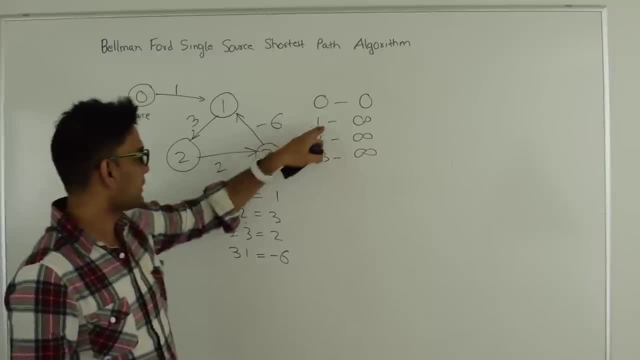 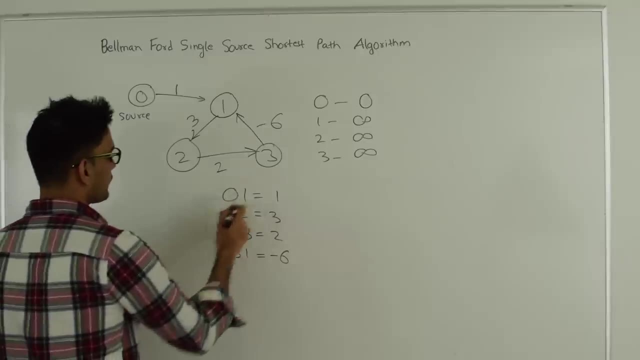 And here the source vertex is 0. So in here all the vertices are at distance infinity, while source vertex is at distance 0. Let's visit the edges in this way, So 0 to 1, this will relax 1. 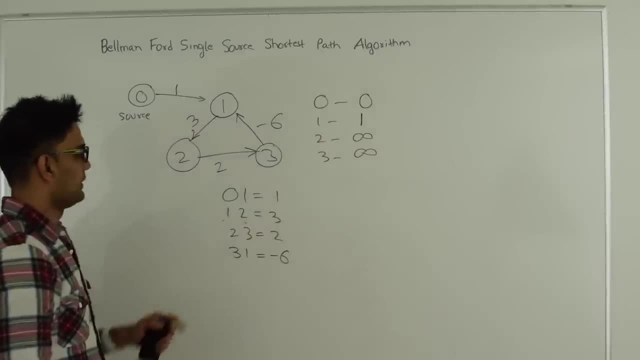 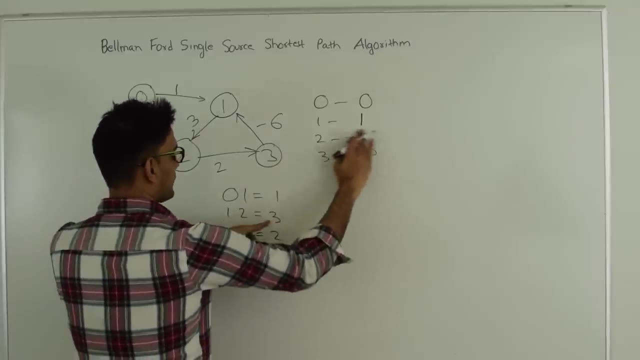 and this will the distance to reach 1 will become 1.. Then we have 1 to 2.. So the distance to reach 2 is infinity, which will be greater than distance to reach 1, which is 1 plus this 3, 4.. 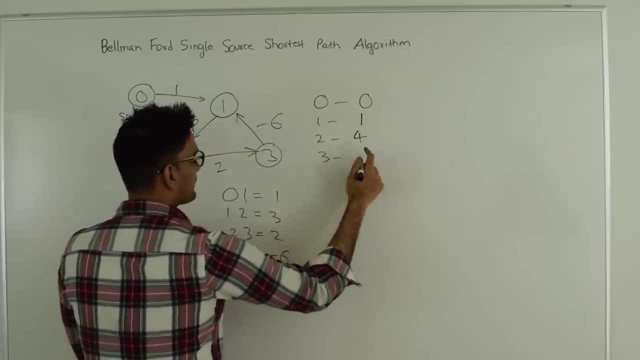 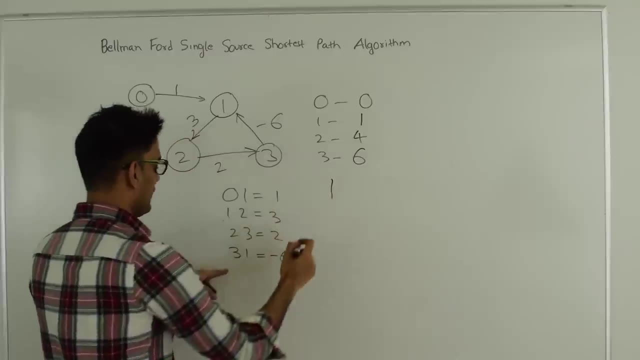 And similarly 3 will be relaxed and this distance will become 6.. And then 3 to 1.. So the distance to reach 1 is 1 right now, And this is going to be greater than the current distance to reach 3. 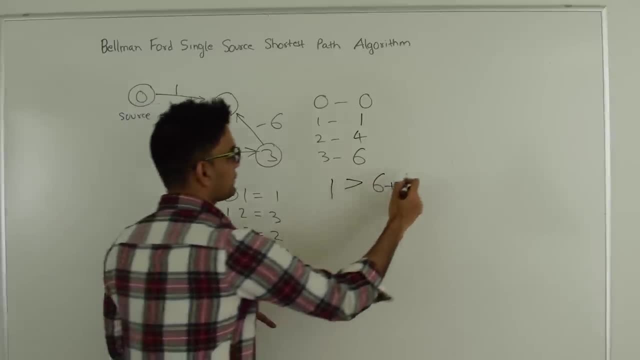 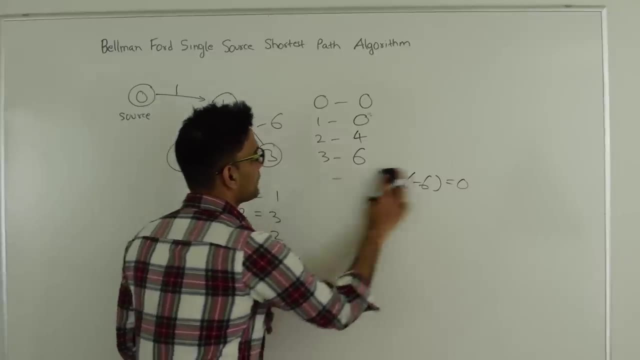 which is 6 plus the weight of this edge, So minus 6.. So basically 0.. So this distance becomes 0.. So this is how the distances look. after one iteration, We have two more iterations to do. 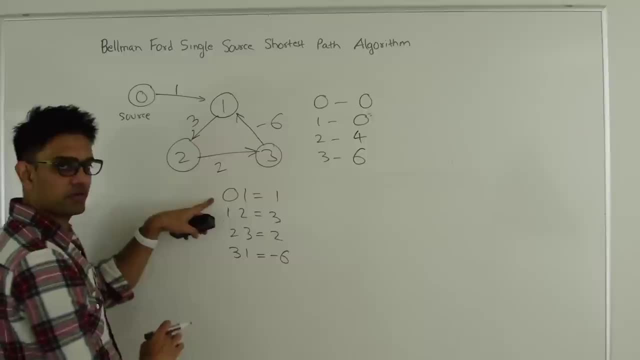 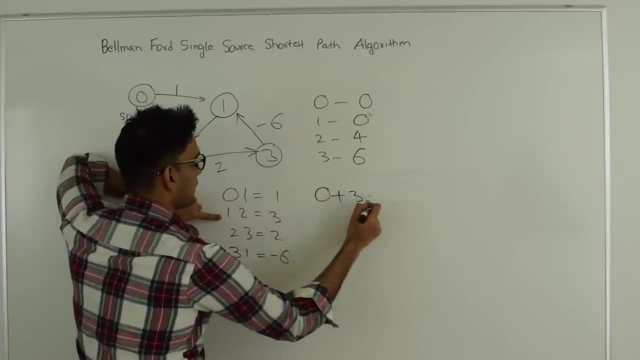 So, going back again, this edge is not going to contribute anything. If we pick this edge, the distance to reach 1 is now 0 plus. the weight of this edge is 3, which is less than the current weight of 4.. 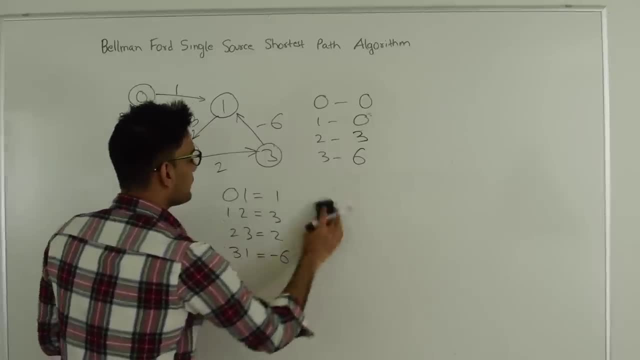 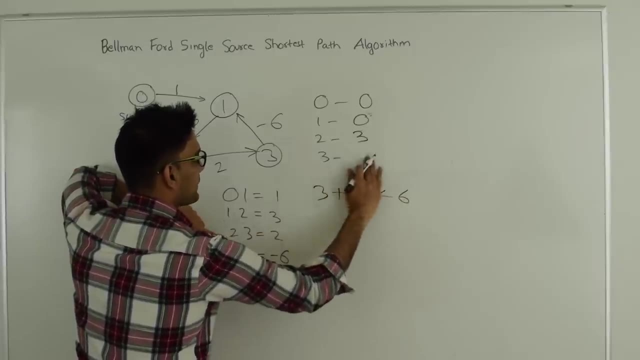 So this becomes 3.. Then distance to reach 2 is 3 plus the weight of this edge is 2, which is less than 6.. So this becomes 5.. And then distance to reach 3 is 5. 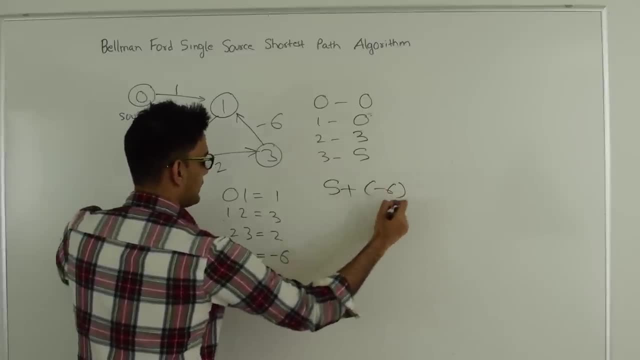 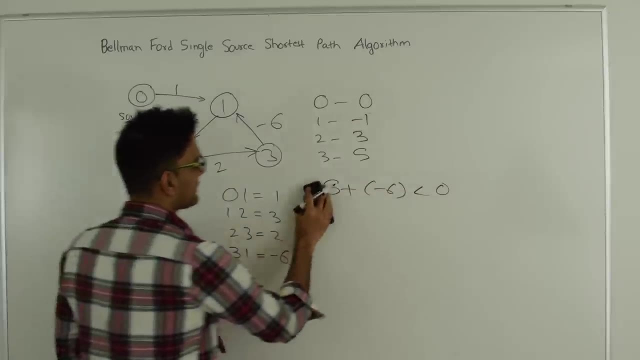 plus, the weight of this edge is minus 6, and this is less than 0. This is minus 1.. So this becomes minus 1.. So this is how it looks. after second iteration, Let's do the third iteration. This is not going to help. 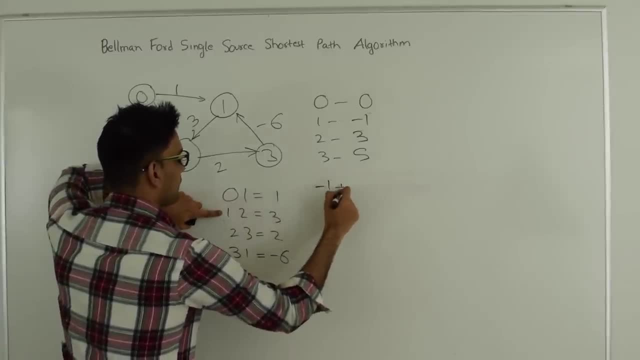 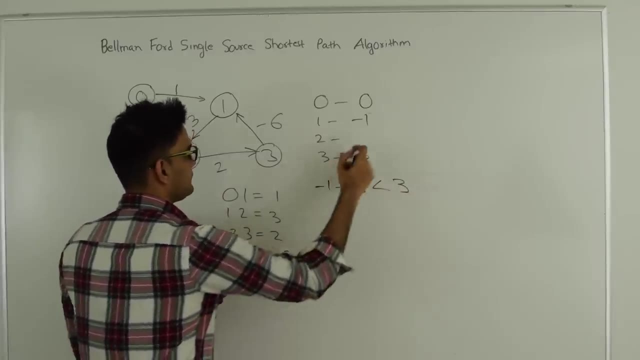 Distance to reach 2 is minus 1 plus. the weight of this edge is 3.. It is less than what we have here, 3.. So this becomes 2.. Similarly, after we do this, relax this edge. this will become 4.. 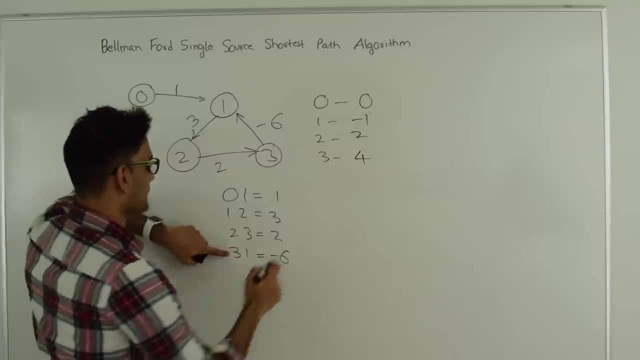 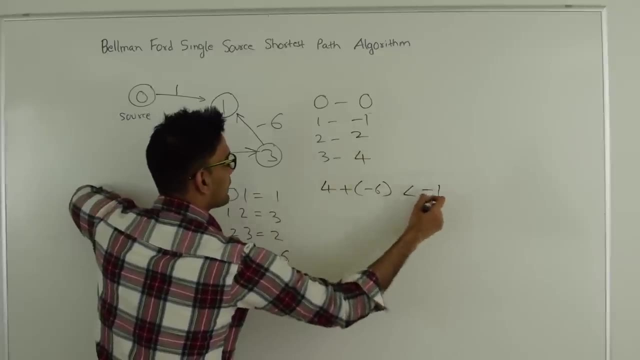 And then, finally, when we relax this edge, the distance to reach 3 is 4 plus minus 6, the weight of this edge, and this is going to be less than minus 1.. So this becomes minus 2.. So, after three iterations, this is how it looks like. 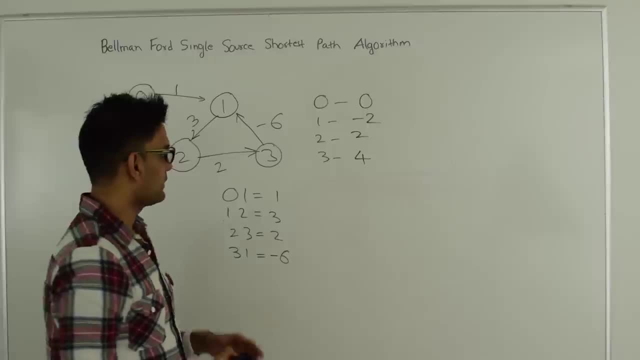 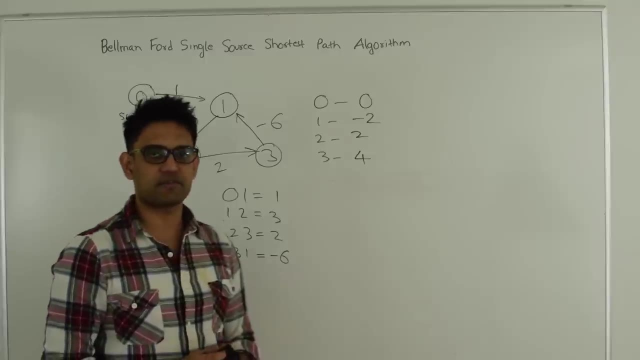 So either this is the answer or there is a negative weight edge in the cycle, Negative weight cycle in the graph, And to find that after v minus 1 iterations we do one more final iteration. Let's do that So, and if the weight 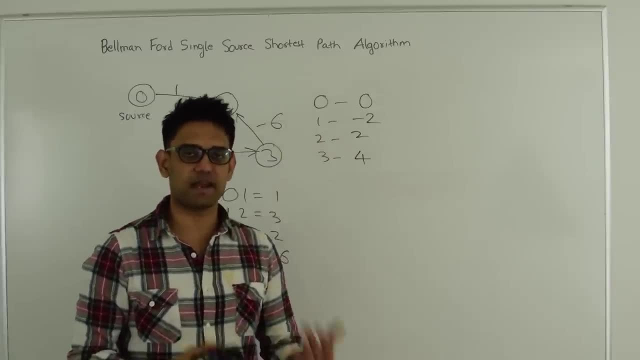 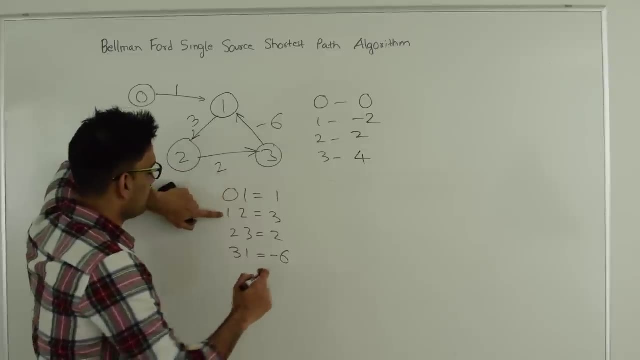 if the distance continues to decrease even in that iteration, it means that there is a negative weight cycle in the graph. So 0, 1 doesn't help 1 to 2.. So distance to reach 1 is minus 2. 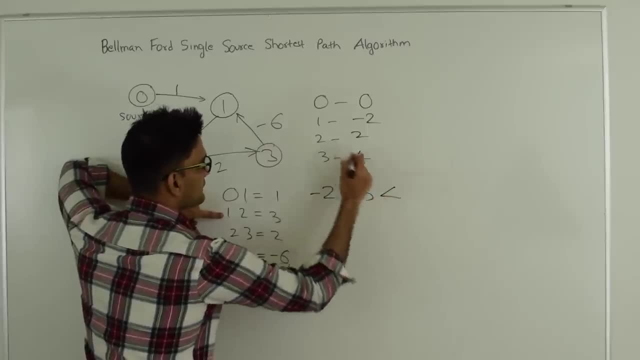 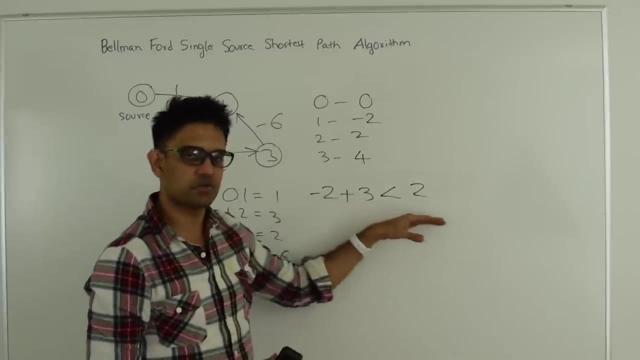 plus, the weight of this edge is 3, and this is less than the current distance to reach, 2, which is 2.. This is 1.. So it means that the distance continues to decrease. So at this point of time we can flag that. 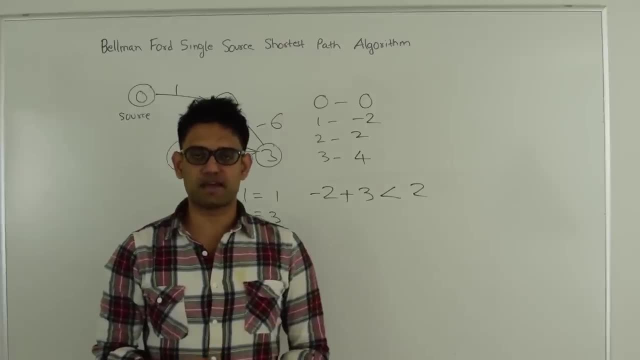 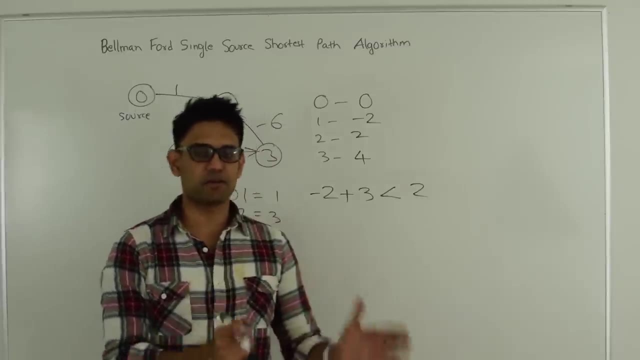 there is a negative weight cycle, and somehow deal with that situation. So this is how Bellman-Ford detects negative weight cycle in the graph: In the vth iteration after v, minus 1 iteration in the vth iteration if the distance continues to decrease. 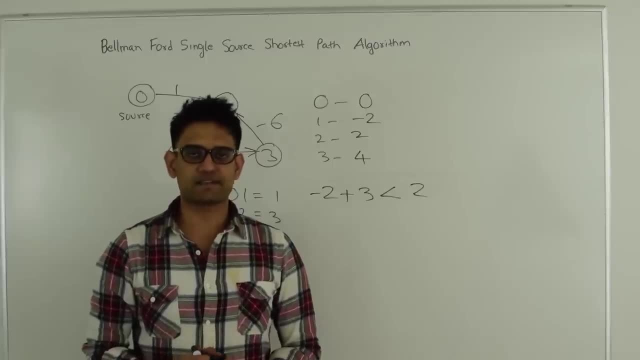 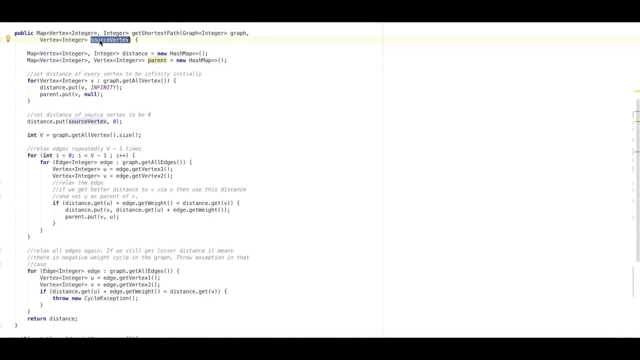 it means that there is a negative weight cycle in the graph. So next let's look at the code for this algorithm. The function is get shortest path. It takes in the graph and the source vertex from which we want to find the shortest distance. 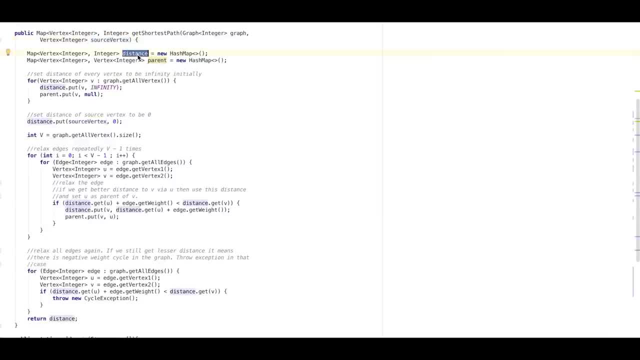 of every other vertex. We initialize two maps- distance and parent- for storing the minimum distance found so far from the source vertex and the parent of every vertex, as we discussed before in the video, And then we are going to iterate through every vertex and then in this distance map. 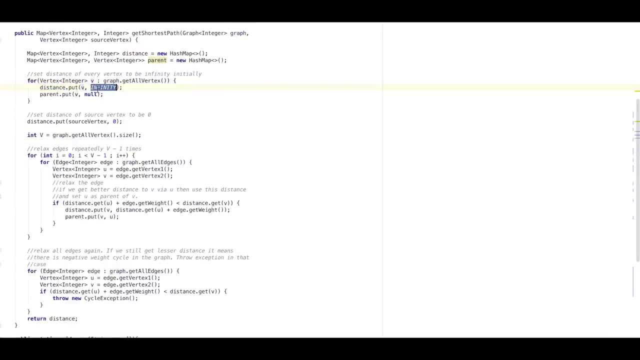 set the distance of that vertex from the source vertex initially to be infinity and set the parent to be null. And then we are going to go to the map and update the distance of source vertex to 0, because it is a distance 0 from itself. 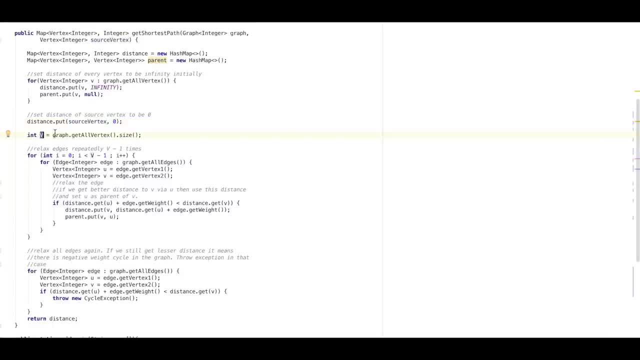 Then I'm going to get this v, which is the total number of vertices in the graph, and then we are going to repeatedly relax the edges v-1 times. So we go for i goes from 0 to v-1 and then we go through every edge. 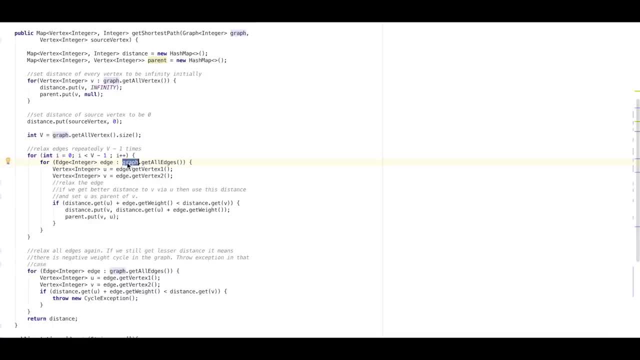 in some every edge of this graph in some random order. get u the start of the edge v the end of the edge and then we relax the edge If distance of u plus the weight of the edge is less than distance of v. 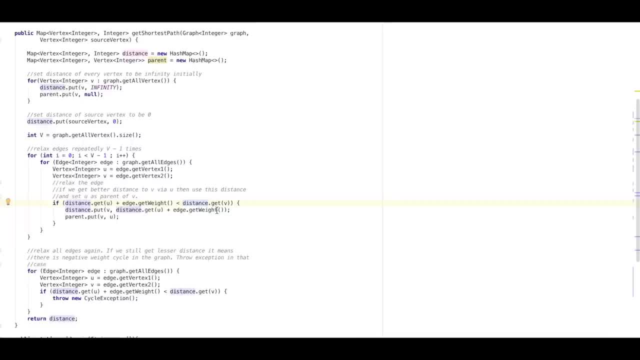 then we update distance of v to be distance of u plus weight of the edge and set the parent of v to be u And, as we discussed before, we repeat this process v-1 times After that, after doing this v-1 time, 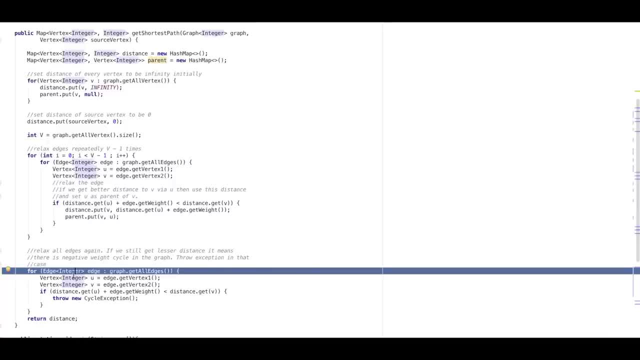 we do this one more. we do this relaxation of all the edges one more time. And in this time, if the distance of any vertex becomes less than what it has already till now, then it means that there is a negative weight cycle in the graph. 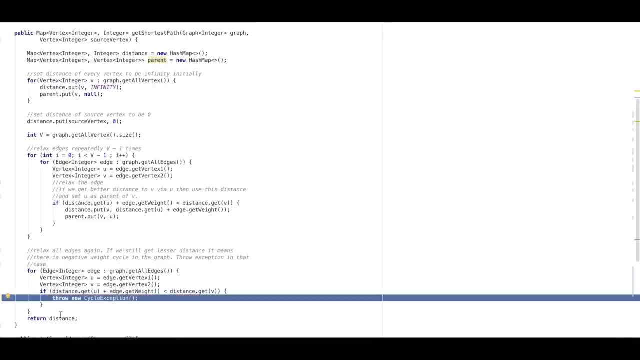 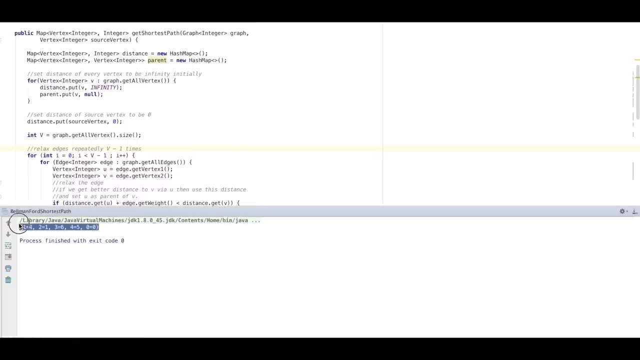 and then we just throw this exception. Otherwise, we just return this distance map, which is storing the distance of every vertex from the source vertex. So let's quickly run this code here. So, as expected, the graph is same as we discussed before.